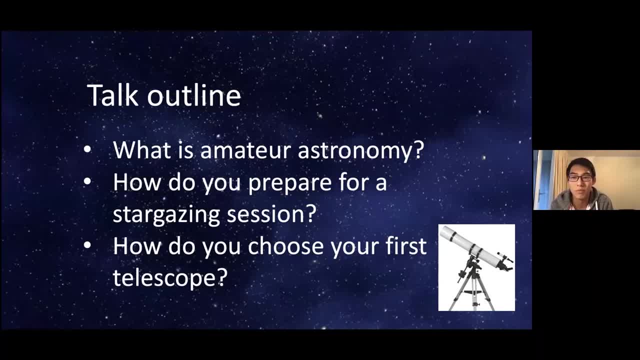 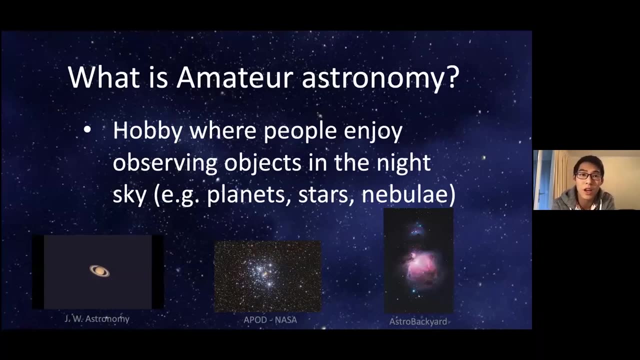 stargazing session. This talk will be about 15 to 20 minutes long and, as I'm talking, feel free to leave questions in the comments below, As I'll be answering them at the end. So what is amateur astronomy? Amateur astronomy is a hobby where people enjoy. 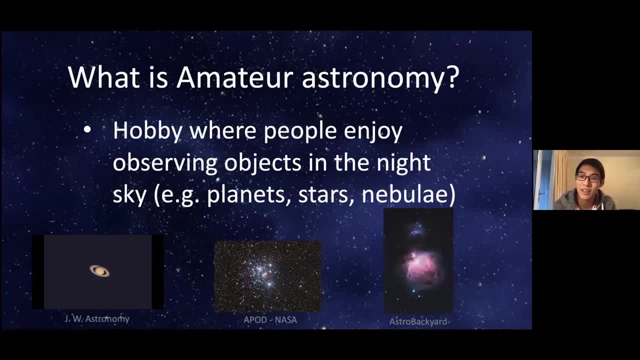 observing objects in the night sky, including planets, stars and nebulae. Why do they do so? It's because they appreciate the beauty of the night sky and they want to spread this passion of astronomy to other people. I could give you many reasons why you should. become an amateur astronomer, but I guess the best way to do that is to become an amateur astronomer. But I guess the best way to do that is to become an amateur astronomer. but I guess the best way to do that is to become an amateur astronomer. 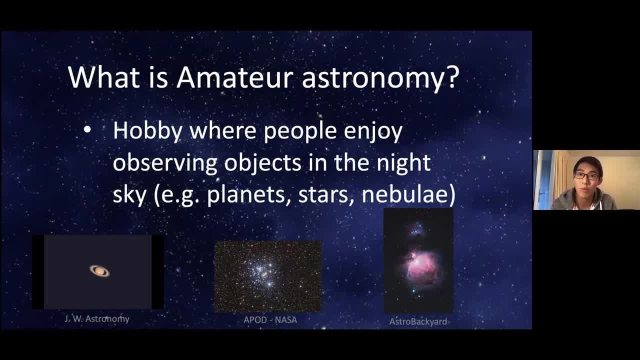 But I guess the best way to convince you is for you to see these amazing objects for yourself. Sometimes the main motivation for amateur astronomy is to take pictures of the night sky, as seen in these pictures below. This is called astrophotography. 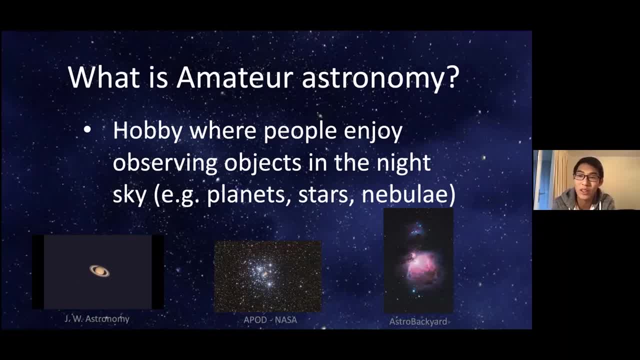 Frankly speaking, there is nothing amateurish about astrophotography, as it can be quite complicated to capture these beautiful images of space. But that is not what I'm going to talk about today. Rather, I'm going to talk about the main aspect of astrophotography. 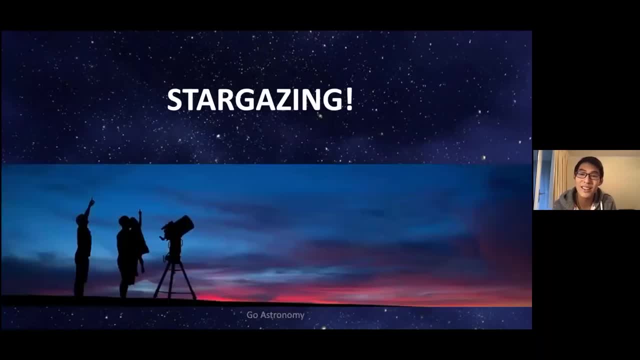 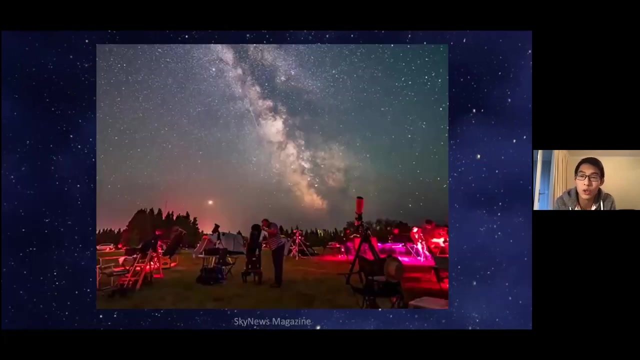 which is stargazing. People all around the world gather to look up at the night sky together, whether is it through the telescopes or just with your naked eye. This can happen in a small group or in a large group through events such as star parties. This creates a sense of 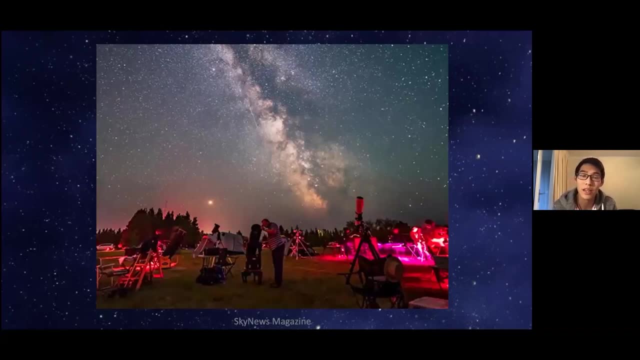 community between the amateur astronomers, all united by the love of the skies. As you can see in this picture over here, it shows the Milky Way, comprising of millions of stars in our galaxy. This is a prominent feature that amateur astronomers love to observe. 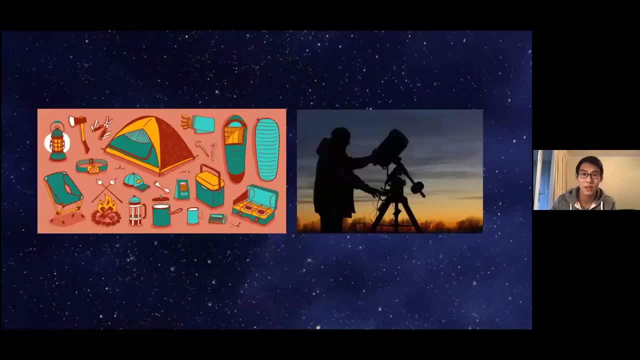 when they are stargazing. While amateur astronomy is essentially about stargazing, doing it isn't as simple as going out to see the stars. Some form of preparation is definitely needed. I like to think of it as going out for camping. 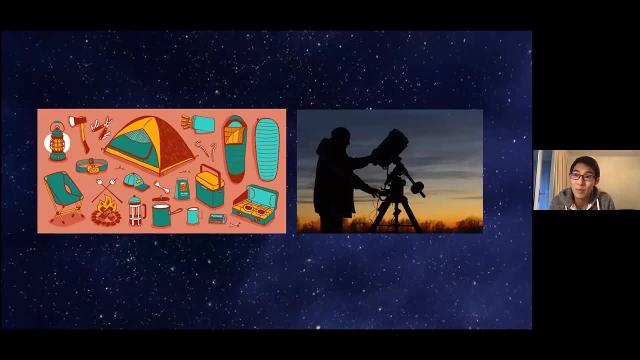 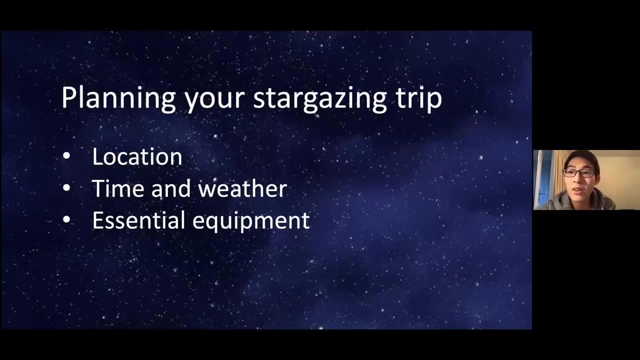 You can't just go out in your t-shirt and a small water bottle. I mean, you can try, of course, but it will not be a pleasant experience. So planning a stargazing trip essentially boils down to these three main aspects: Location, time and weather, and essential equipment. 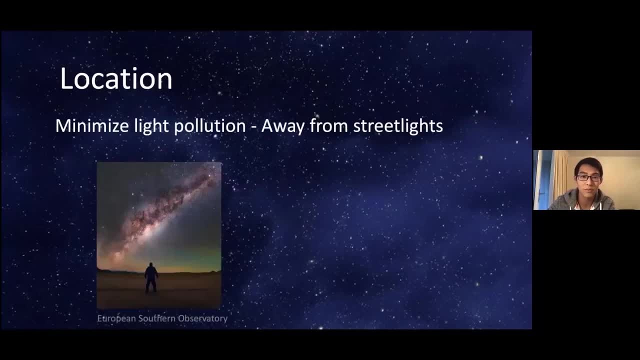 Let's look at the first one location. So it goes without saying that an ideal stargazing site should be dark enough to see the stars. You should aim to be far enough from the city such that the street lights do not outshine the stars in the sky. 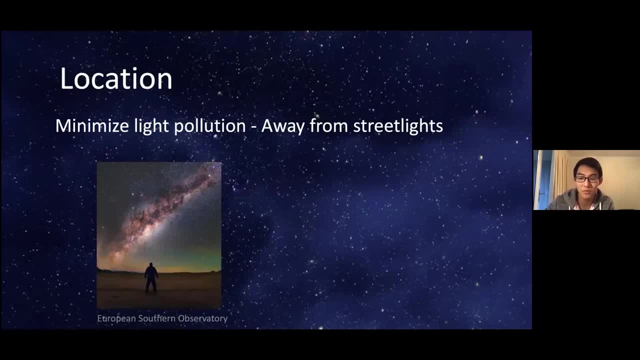 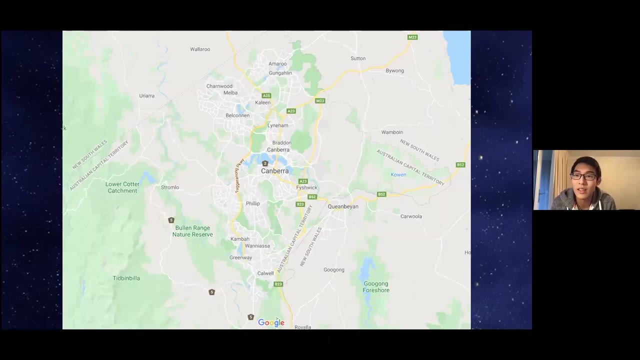 This is commonly known as light pollution. Thus, you do not want to be at a site that is similar to the picture on the right, which shows a significantly light polluted area. To understand this better, let's use Canberra as an example. If you're living here, you're pretty fortunate that the 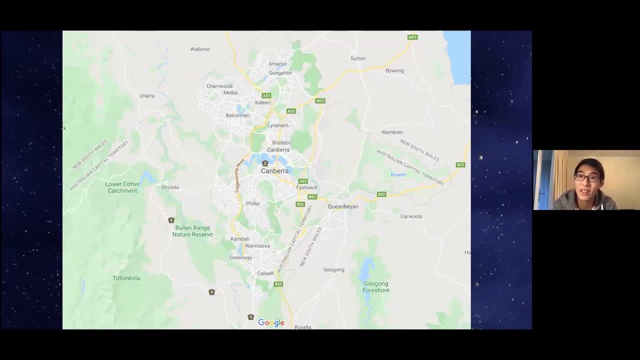 nearest dark skies are not too far away, some even accessible within 15 minutes by car. of course, The areas circled in red show places with a larger density of residents, which means that there will be more light pollution in those areas. Of course, it doesn't mean that you. 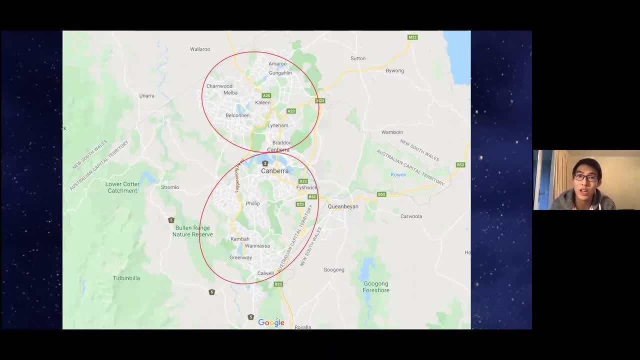 won't be able to see any stars at those locations, but it just won't be as dark as a more secluded location where the Milky Way will be much more visible. Some examples of good stargazing spots, as shown in the arrows, include the east and west. 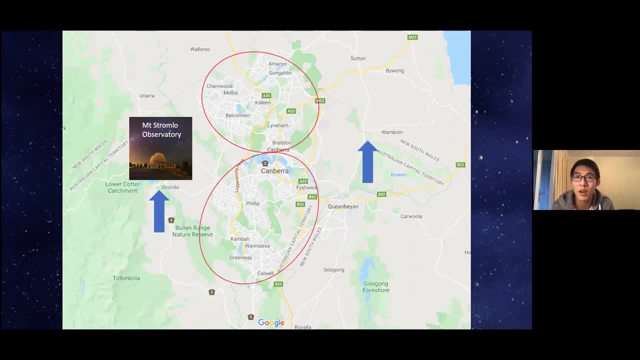 sites of Canberra. One of them is at the Mount Stromlo Observatory, which is why we strongly encourage you guys to join us for our public astronomy nights when this COVID-19 situation is over. of course, If you're feeling a little more adventurous, you might want to try going. 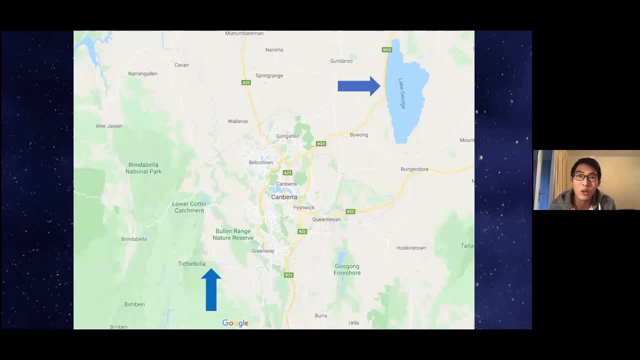 further out to Lake George or Timin Dila, which is a very popular tourist destination. Also, you might want to take a look at Lake George, which offers even better skies than the ones mentioned earlier. For example, this is a photo of the Milky Way taken at Lake George. 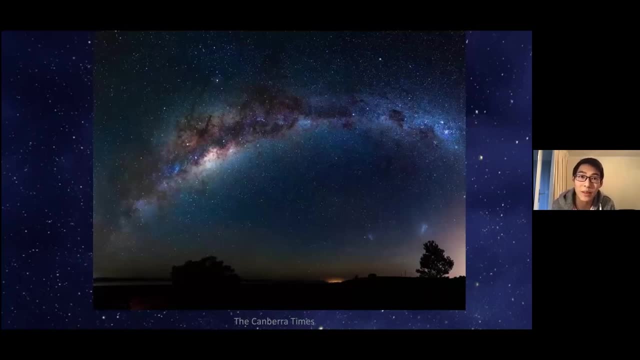 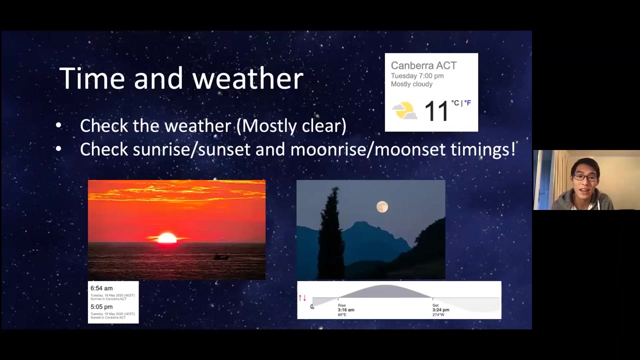 As you can see, there isn't much light pollution to interfere with the starlight. That is why it's an excellent stargazing spot. Again, just a reminder: if you have any questions, do leave them below in the comments. Another thing you should consider when planning a stargazing trip: 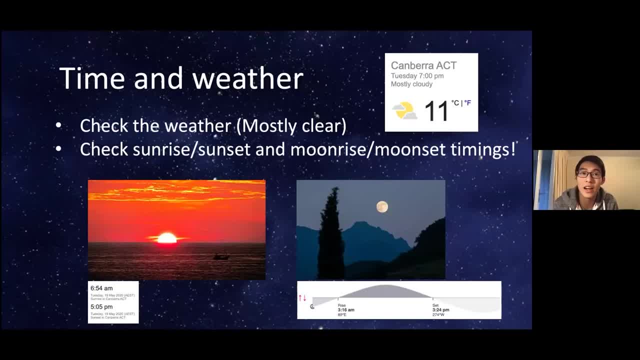 is the time and weather. Make sure you have mostly clear skies before you go out. Looking at today's weather forecast, unfortunately it doesn't look very promising because it's mostly cloudy. It is also important to check the sunrise and sunset timings before you go. 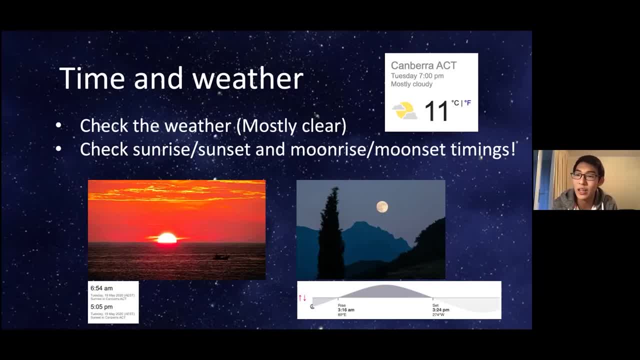 out. This is because we live in a seasonal country and the timings will vary considerably In winter. since sunrise is earlier and sunset is later, you will get a longer duration of dark skies, And the opposite is true in summer. Additionally, you should also pay. 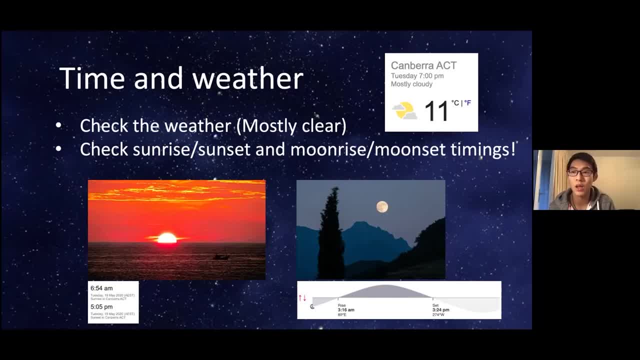 attention to the moon rise and moonset timings. Most beginner astronomers tend to forget this, but the moon really plays a big role in terms of the quality of the dark sky that you get. Even if you are in the most secluded spot possible, if the moon is up, you will ruin your your stargazing experience because it 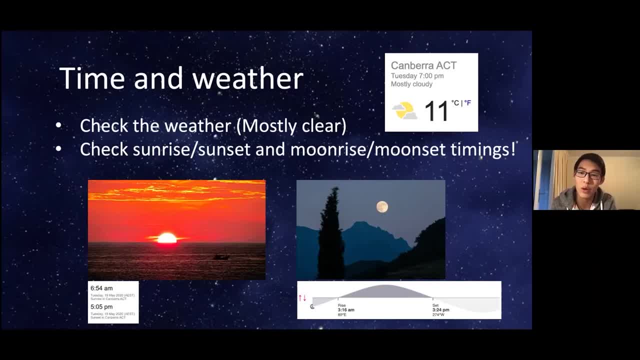 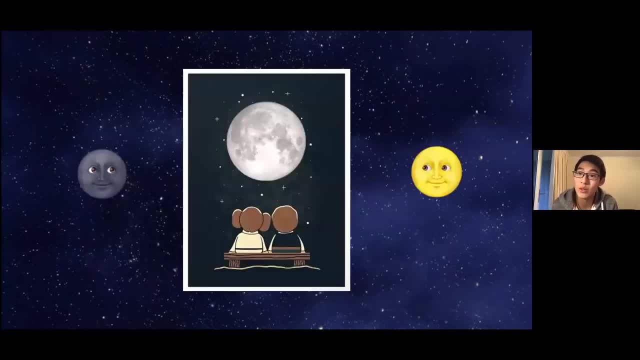 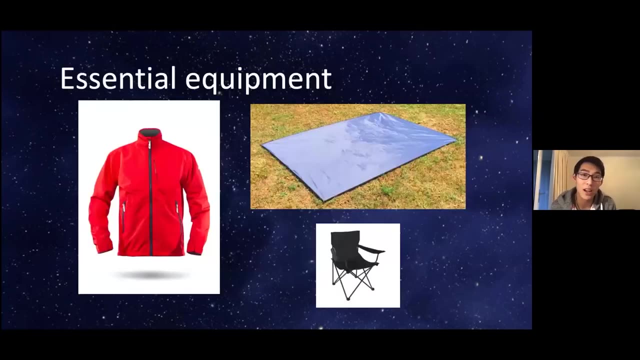 blocks out most of the stars in the sky, including the Milky Way. That is the reason why it is not advisable to stargaze when the moon is up, unless the moon is what you want to observe. Moving on to the essential equipment for your stargazing trip, 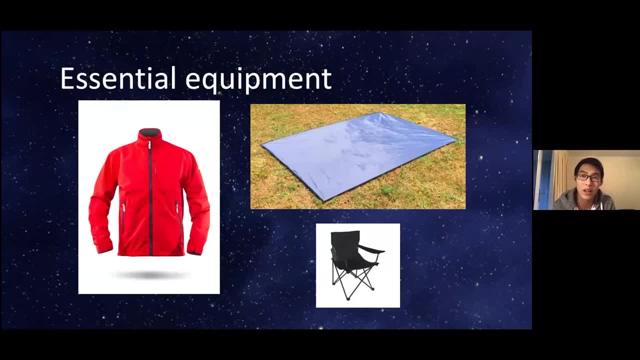 you should make sure that you dress warmly and comfortably, as it will get cold, especially during winter. Also, as you will most likely be in the open, bring a camping chair or, even better, a waterproof ground mat so that you can lie on the back. 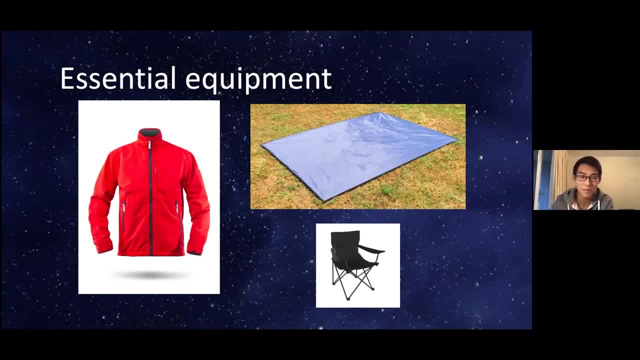 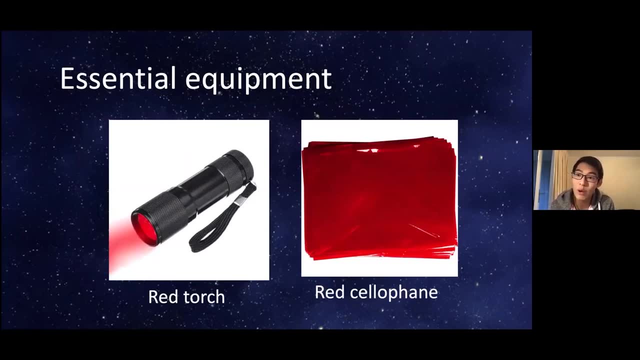 and have a perfect view of the stars. It is also advisable to bring a red torch. You might wonder why red? It is because when you stargaze, your eyes need around 30 minutes to be adapted to the dark so that you can see as many stars as 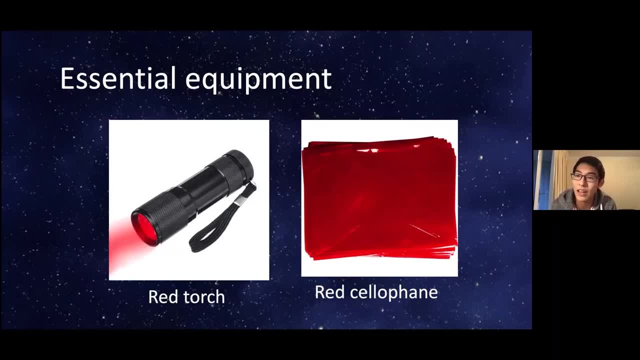 possible. When you use white or other individual colors of light, it will ruin your dark adaptation. Red is the only color that will have the least effect on your eyes. If you don't have a built-in red torch, that is fine, because you can simply put. 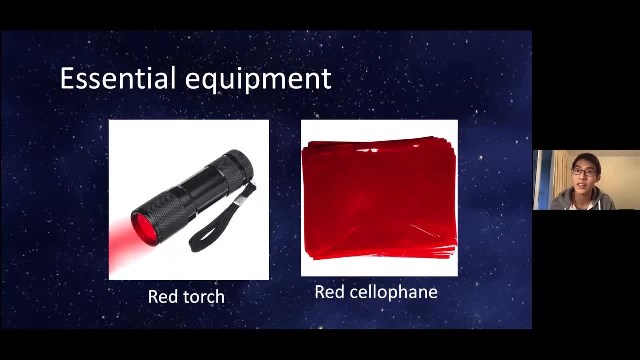 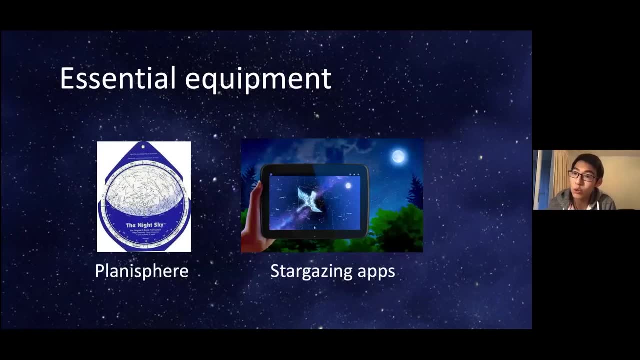 a piece of red cellophane over a white torch and you will be able to see the stars, And that will work as well. Next up for essential equipment are tools that will allow you to navigate around the night sky. On a clear, dark night, it is easy to be. 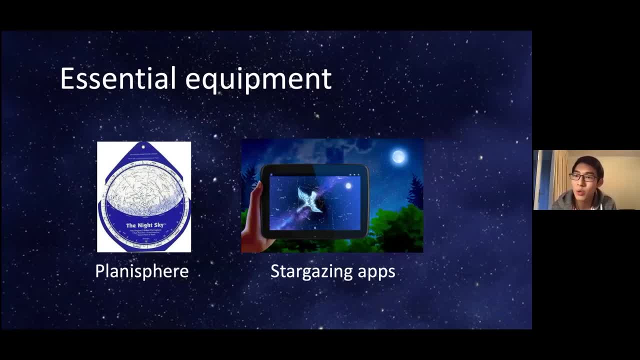 overwhelmed by the number of stars that you see, until you are unsure of what you are looking at. Fortunately, you can either use a planisphere, which is a physical star chart that you can bring around, or stargazing apps on your phone, which are more commonly used today. 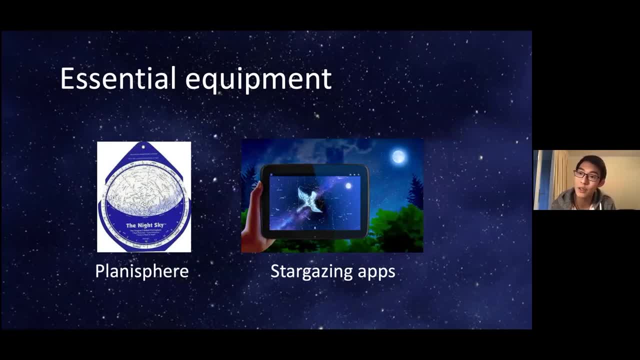 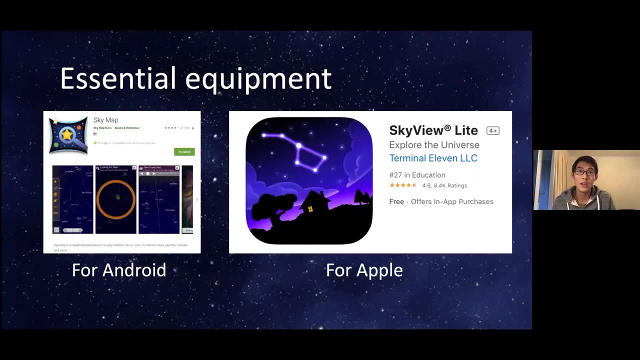 All you need to do is to key in your location and time into your phone after you have downloaded the app, and you can start using it to identify the objects that you are looking at. These are the two popular stargazing apps being used and the good thing about. 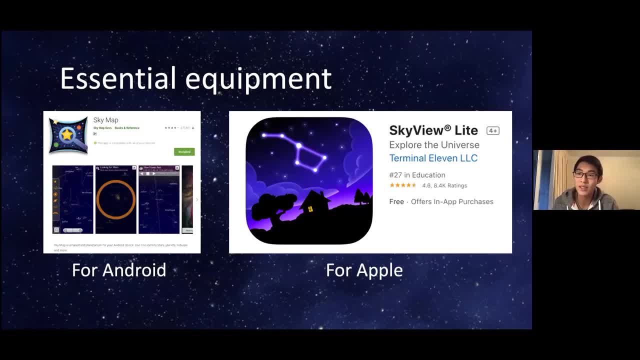 them is that they are free For Android users. SkyMap, also known, and most previously known, as Google SkyMap, is a great tool to use for stargazing, And for Apple users, you can download Skyview Lite. Even though it's just the basic version, it's good enough for you to learn about. 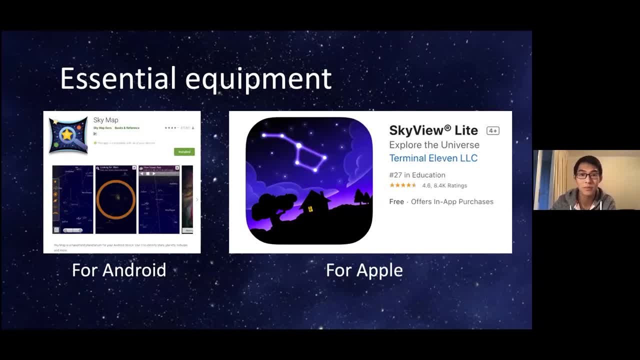 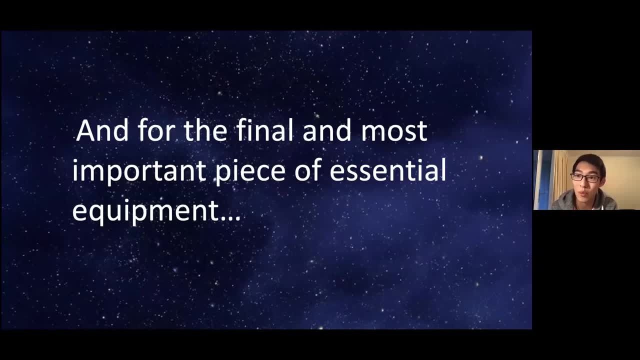 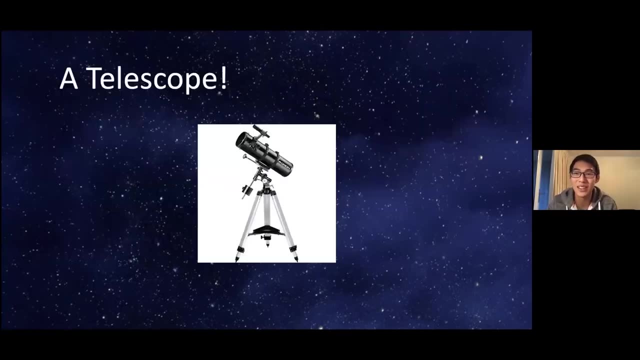 objects in the night sky. And for the final and most important piece of equipment that you need for stargazing, which some of you have been waiting for. yes, I'm referring to hot chocolate and cookies, Just kidding, I'm actually referring to a telescope. 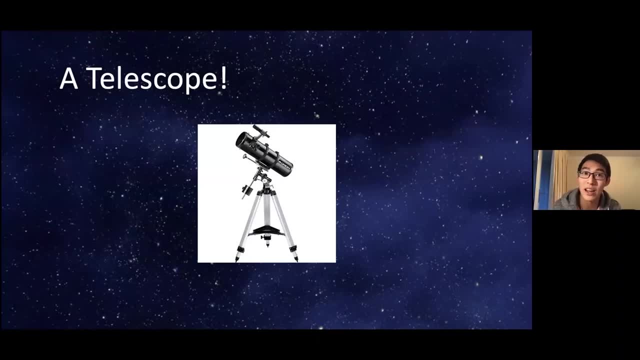 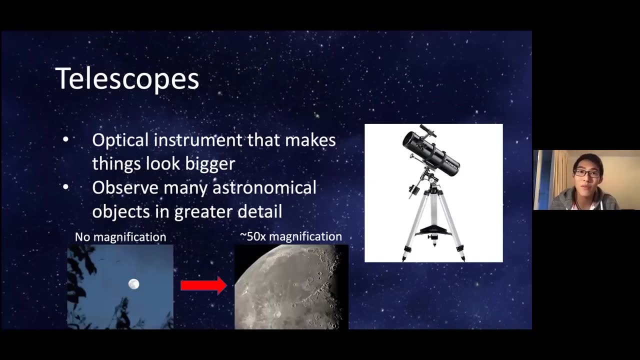 So what does a telescope do and why is it important for stargazing? Well, a telescope is an optical instrument that makes objects look bigger, which is great for stargazing, because it can help you see objects in the night sky, Most of the things that we want to observe in the night sky. 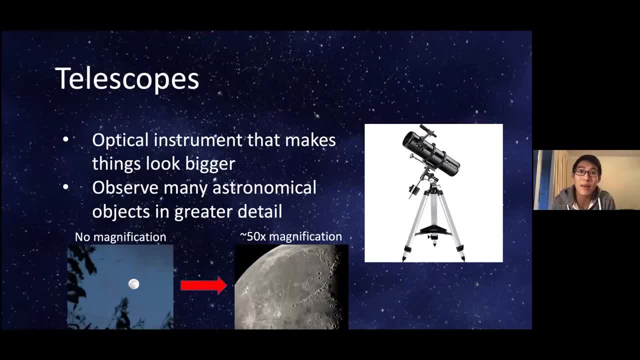 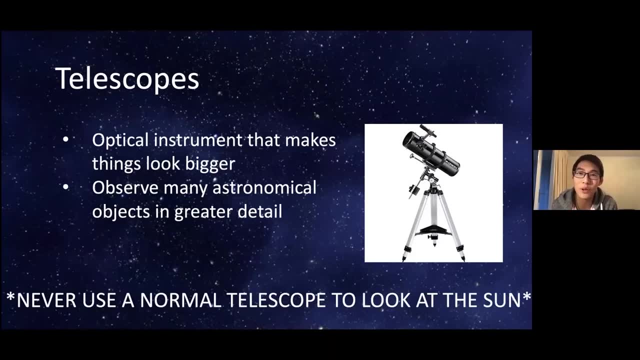 are distant and tiny, so this allows us to see them in greater detail, such as the moon below. Also, an important safety reminder for you guys is to never use a normal telescope to look at the sun, as it might cause you to go blind. 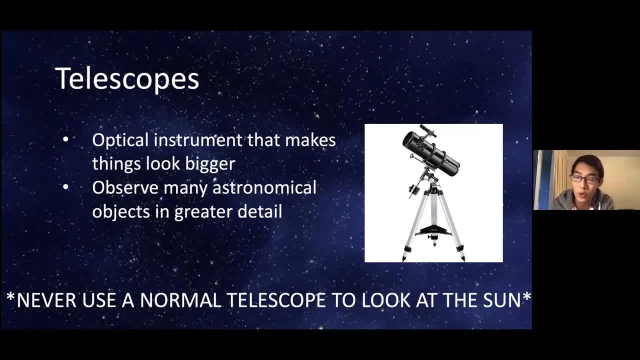 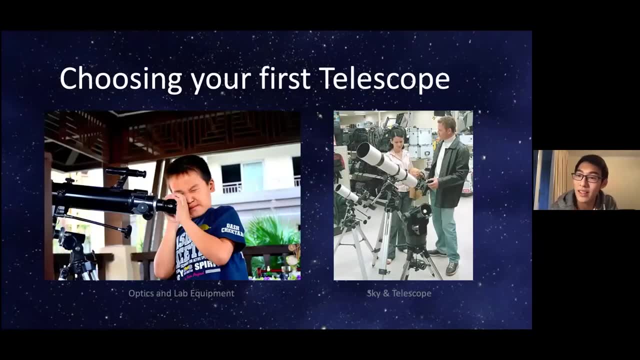 If you want to look at the sun, there are special solar telescopes for this purpose. Now getting your first telescope can be an exciting yet daunting time, regardless of your age, And it's understandable, because most telescopes cost a few hundred dollars. 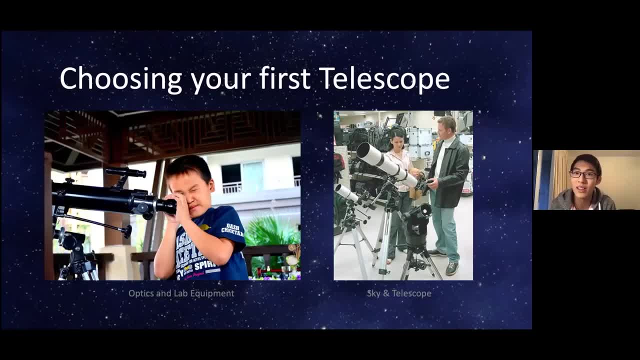 and the last thing you want to do is to invest in something that you only use once, be disappointed and then store it away forever. So what I'm going to do is to give you some important guidelines that you can consider when you are about to get your first telescope. 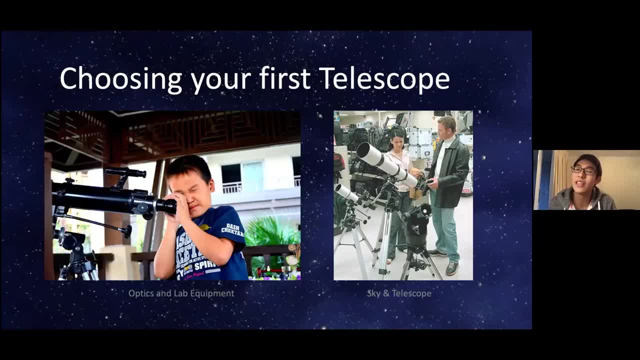 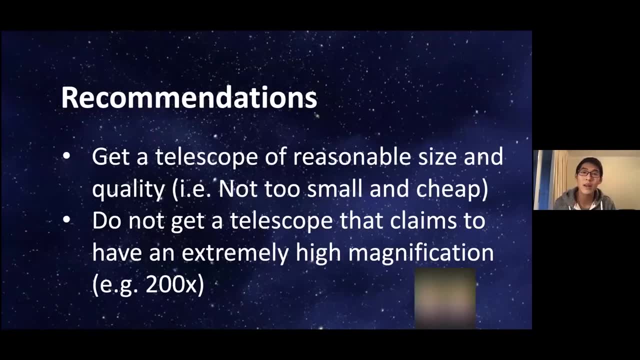 I'm also going to give some recommendations, but these are definitely not exhaustive, as there are many good telescopes out there. Here are some guidelines when it comes to choosing your first telescope. Try to get telescopes of reasonable size and quality so that you get the most out of your stargazing experience. 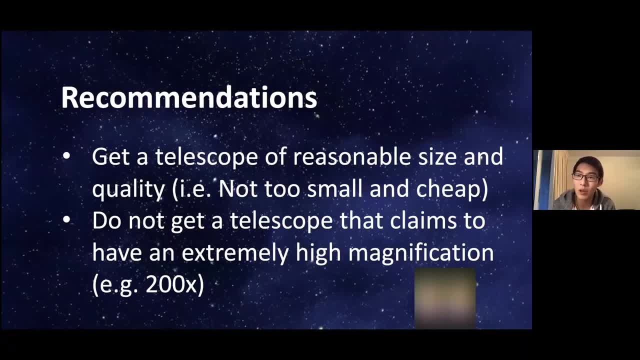 When you get a cheap telescope, the danger is that the quality won't be great. Sure, you might be able to observe the moon and some planets, but a plastic build, cheap lens and unstable tripod will most likely not allow you to observe anything else. 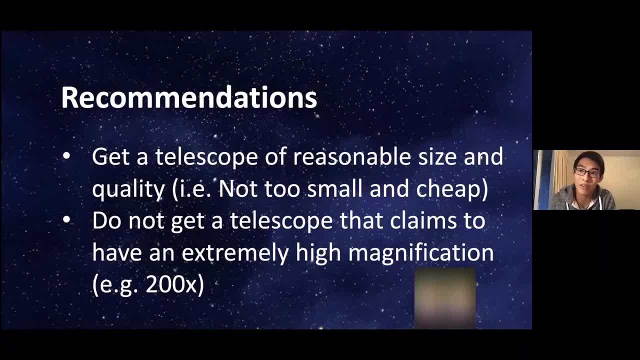 Also, don't get a telescope that claims to have an extremely high magnification, such as above 200. Why is that so? When you increase the magnification to an extreme amount, it's harder to focus and the amount of light reaching your eyes decreases sharply. 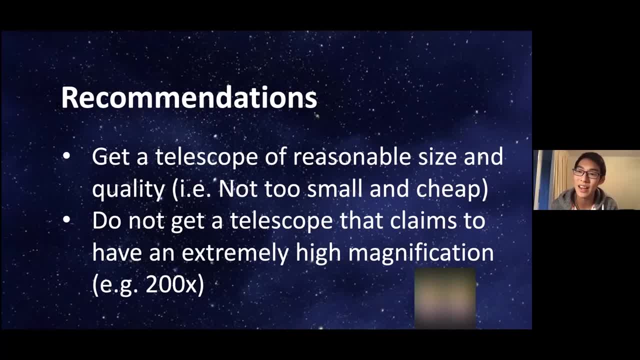 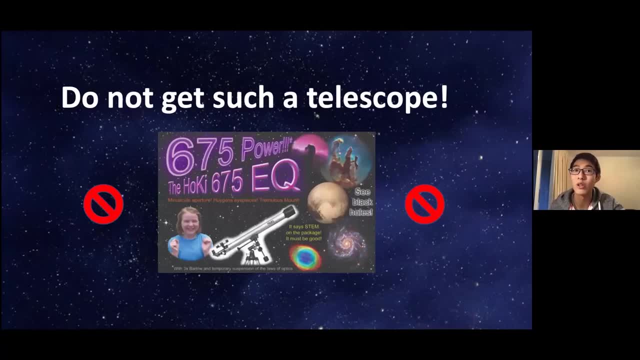 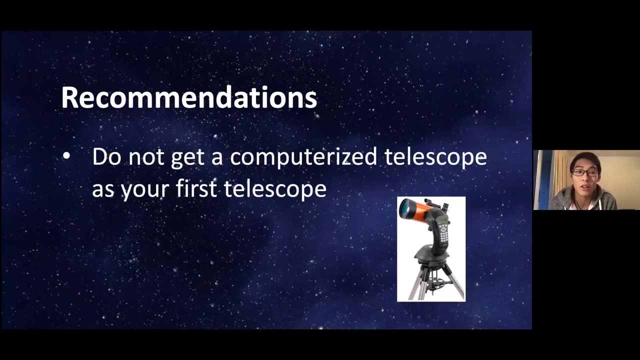 and all you get is just a sad blurry blob. So this ad over here is an example of a telescope that you should never, ever get. It is also recommended that you don't get a computerized telescope as your first one. For those who are unfamiliar with the telescope: 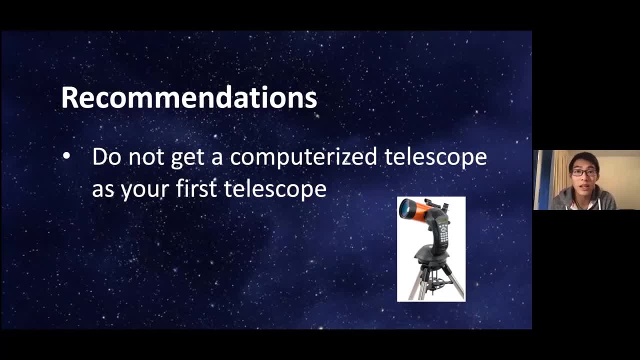 you can get a computerized telescope, but if you aren't familiar with this term, a computerized telescope is one that is able to find and track the objects for you with just a push of a button. If it's such a cool and convenient piece of equipment, 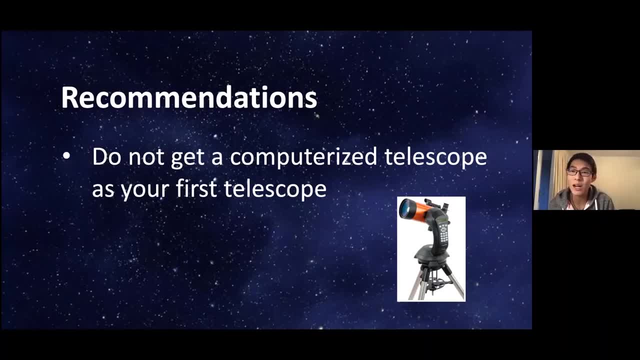 why am I telling you not to buy it? Firstly, it's much more expensive than the manual ones- at least twice the cost. But more importantly, it defeats the purpose of familiarizing yourself with the night sky. From personal experience, the satisfaction of finding the objects yourself using a manual telescope is much greater. 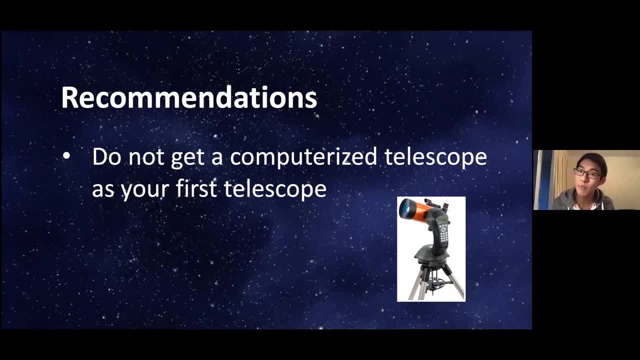 even though it may be challenging at the start, And you can even point out the objects that you're observing to others. The only reasons, in my opinion, the only reasons why, the only reasons that you should get a computerized telescope is when you're organizing stargazing parties. 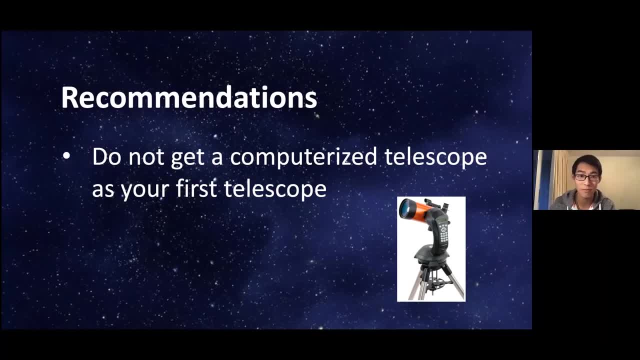 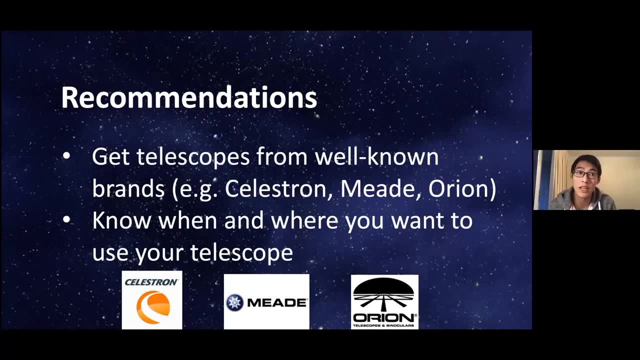 or when you need it for astrophotography. Therefore, you should get telescopes from well-known brands such as Celestron, Mead and Orion- And of course, there are many more- And you should know when and where you want to use your telescope. 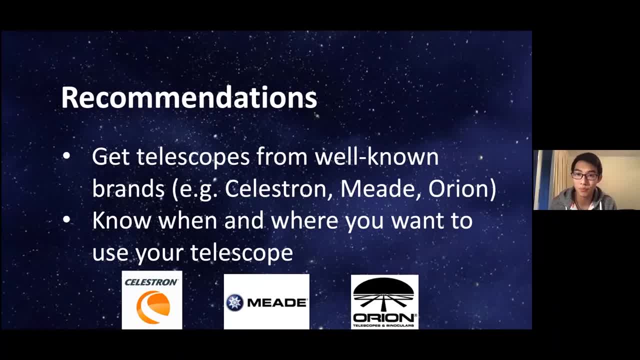 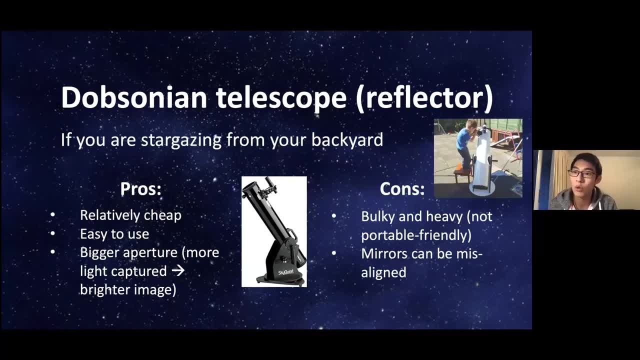 as it will greatly affect the kind of telescopes that you should get. So if you are stargazing from your backyard, and since it's relatively dark there and you don't see, a point of traveling for your stargazing trips. 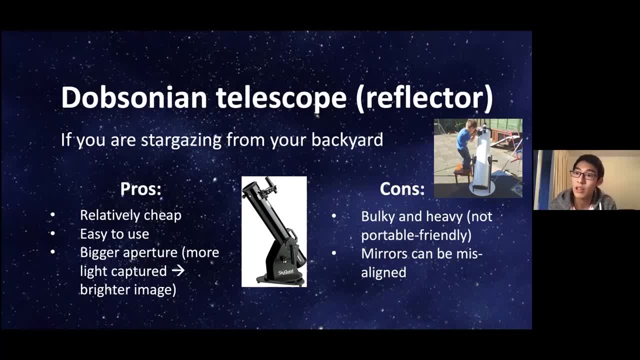 you should get a Dobsonian telescope. A Dobsonian telescope is a reflector that uses mirrors to magnify the image. The pros are: it is relatively cheap, it's easy to use and it has a bigger aperture, which means it captures more light. 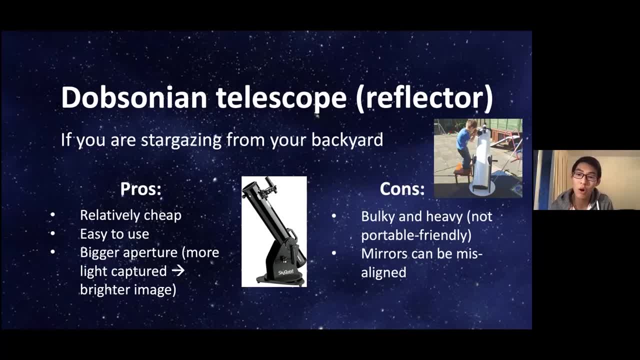 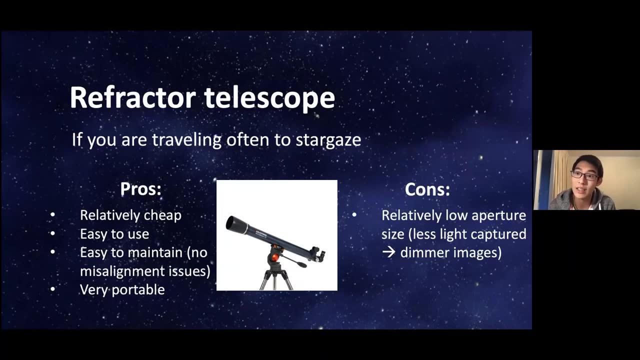 and has a brighter image. However, the cons are: it is bulky and heavy, not portable friendly, and the mirrors can be sometimes misaligned. Now, if you're traveling often to stargaze and portability is an issue, you should consider getting a. 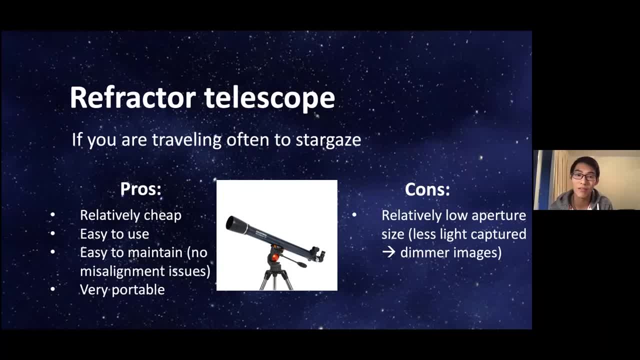 refractor telescope which uses lens to magnify the image. The pros are: it is relatively cheap, it's easy to use, just like a Dobsonian telescope, but it's also easy to maintain because there are no misalignment issues with the mirrors. 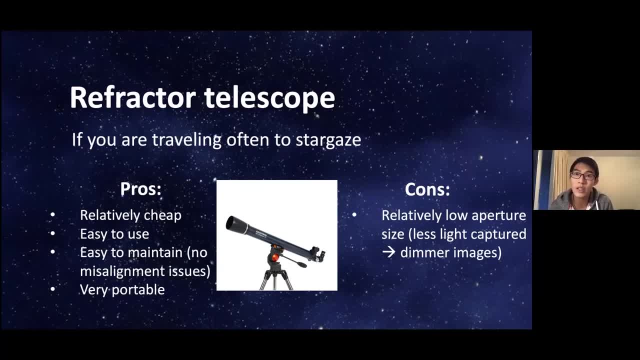 and it's also very portable. However, the cons are it has a relatively low aperture size, which means you get a slightly dimmer image. So if you're not ready for stargazing, you should get a Dobsonian telescope. So if you're not ready for stargazing, you should get a Dobsonian telescope. 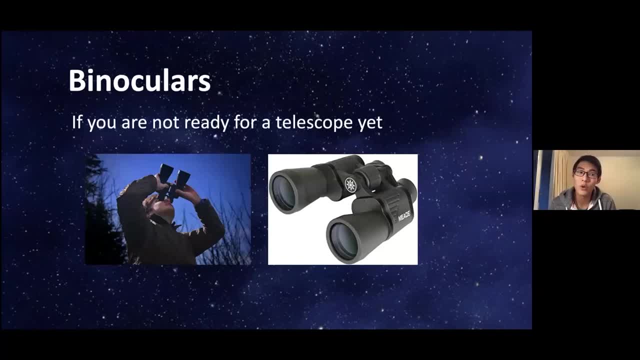 If you're not ready for telescope yet, there is still an option for you: You can consider getting a pair of binoculars. The good thing about binoculars is that it's much cheaper and portable than a telescope, due to its low weight. 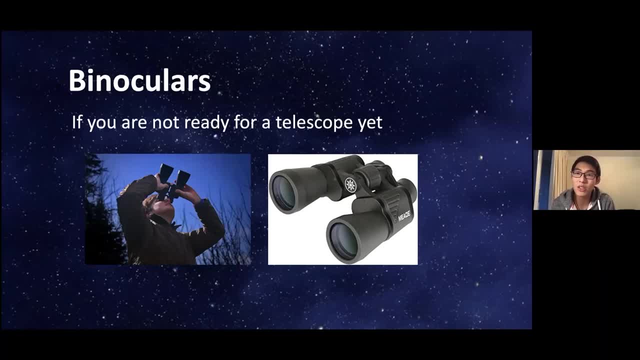 which means that you can easily hold it in your hands. Because of its lower magnification, you can also simply use it to scan across the sky to look for interesting objects. Even till today, I sometimes bring a pair of binoculars out for stargazing. 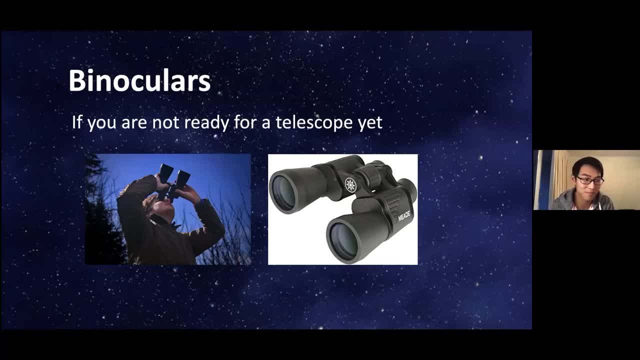 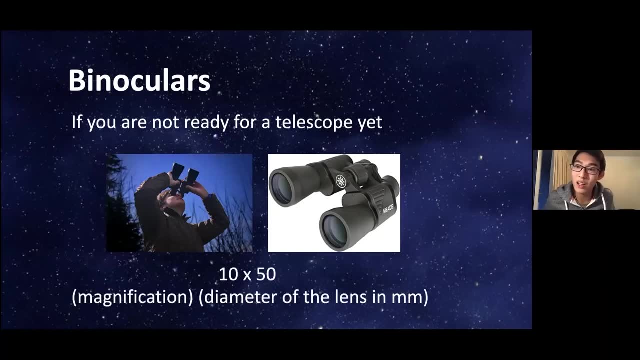 instead of telescope due to its convenience. I will also share another reminder that I keep in mind, in case there's not enough information for my people to know how to use the binoculars. Before I move on, Another reminder to leave questions below. 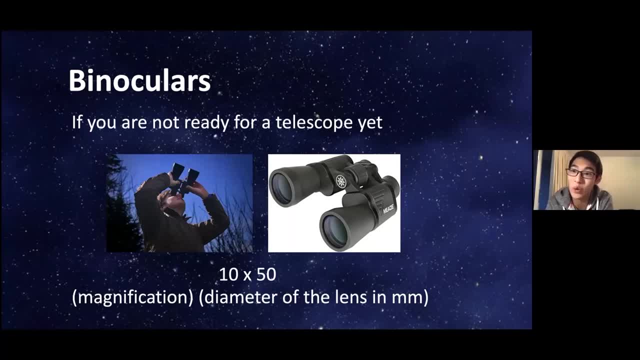 so that I can answer them at the end during the Q&A session. An example is this: Share some tips when it comes to buying a pair of binoculars. You might find that binoculars are usually described by two numbers. The first number represents magnification. 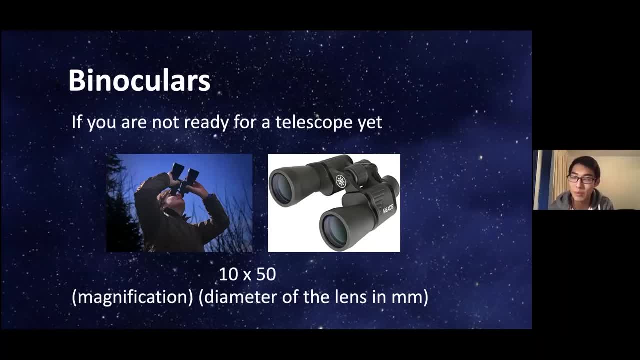 While the second number represents the diameter of its lens in mm- We can let it know that beginning the start is soon- And the first number represents the millimeter of length of the lens In mm, which is 2225.. You may have done some research before, though. 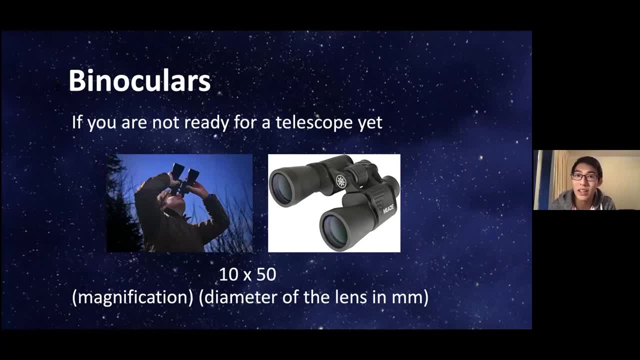 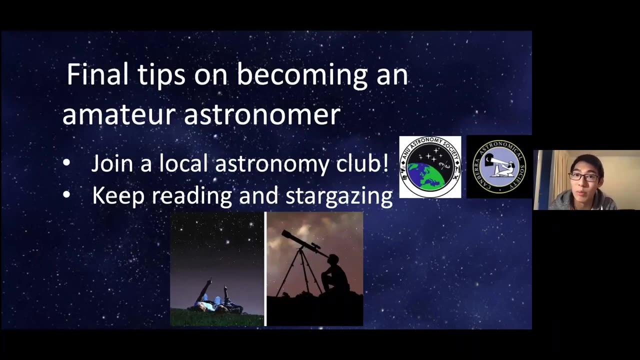 The 10 by 50 configuration is highly recommended if you want to have a good balance between magnification and brightness. To end off, here are some final tips on becoming an amateur astronomer. As I've mentioned before, amateur astronomy is about sharing this passion and hobby. 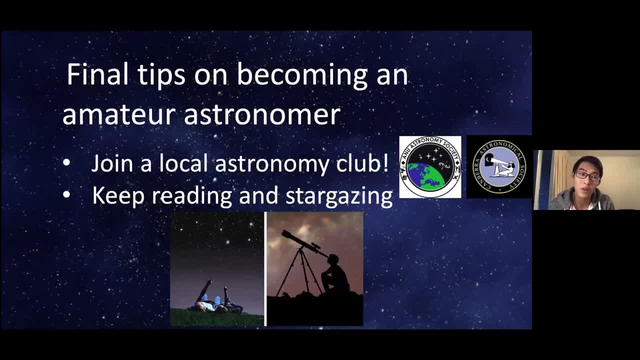 with the rest of the community. That is the reason why you should join a local astronomy club when you can. The two clubs I know in Canberra are the ENU Astronomy Club as well as the Canberra Astronomical Society. By joining these clubs, you actually get a chance to interact with experienced 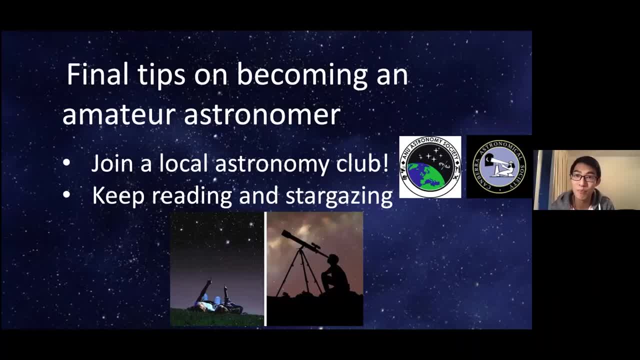 amateur astronomers as well as learn a thing or two from them. Another thing would be to keep reading and stargazing. What I've covered today is just the tip of the iceberg, and there are still lots of things to learn in astronomy. Fortunately, we live in an age where 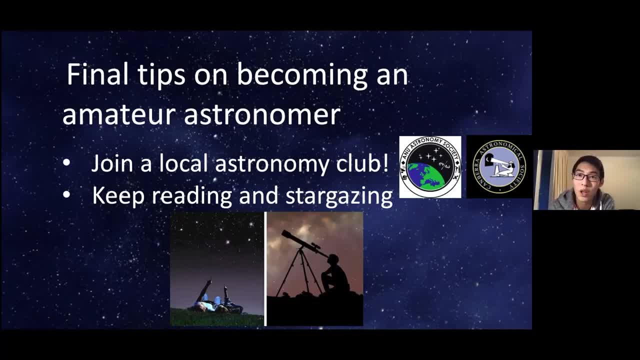 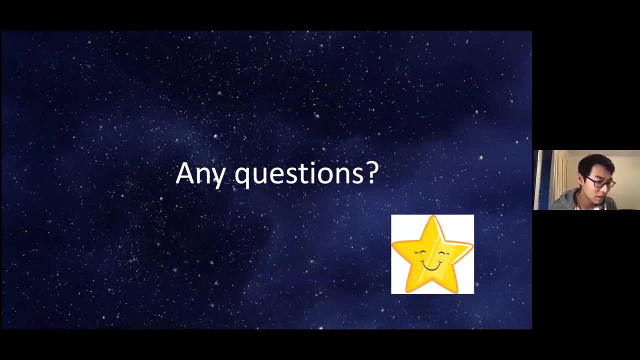 there is plenty of information on the internet as well as in books. With patience and some determination, this hobby can grow into a wonderful journey of a lifetime. With that, I thank you all for listening to my talk. Any questions? Yeah, so we will wait and see if there are any questions, otherwise we will wrap. 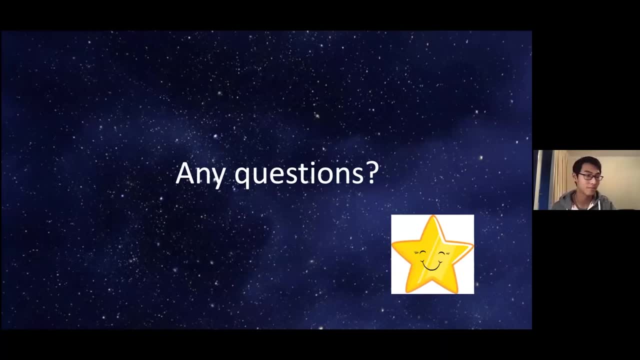 this talk up. Thank you very much. Um, I think I didn't emphasize this enough, but when it comes to choosing a telescope, the brightness of the image is actually more important than the magnification, as I mentioned. So the brightness is like you should get um the minimum size of the telescope. uh, 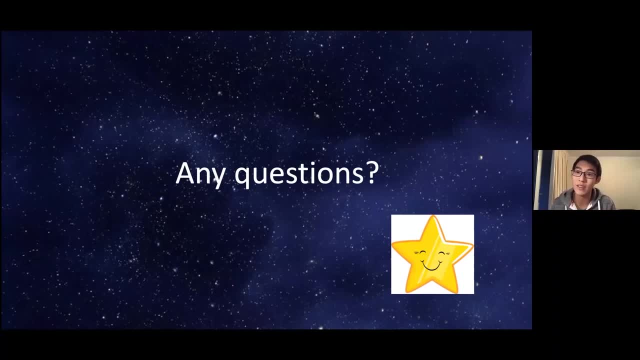 should be around three inches, which is about 75, um 75 millimeters. sorry wait, is that correct? Yeah, It's about three inches, So the diameter of the lens or the diameter of the aperture should be at least three meters. 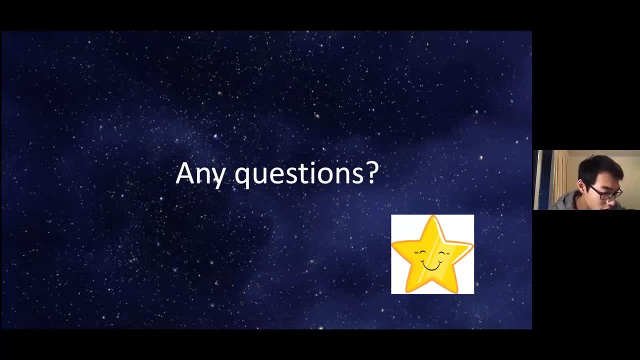 in openings. Okay, We have uh one question, uh, more info about. so, okay, When it comes to telescopes, um, they actually, um, I would say, three different types of telescopes. Um, you have, I've mentioned the reflector, which uses mirrors. 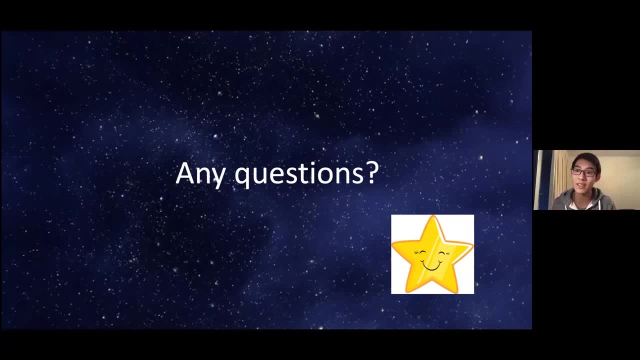 There's also a refractor with which uses lenses, And there's also the last type which I didn't mention in the talk just now is called catadioptrics. So catadioptrics is um is a very special optical instrument. 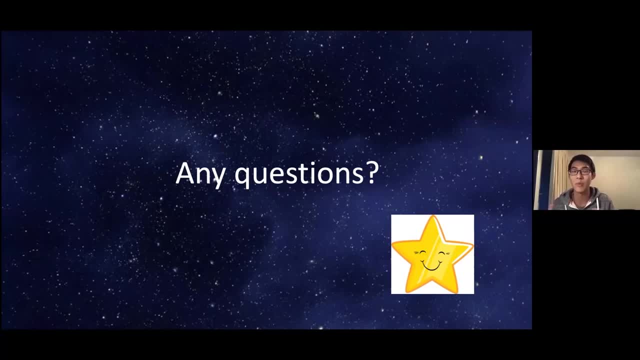 Which uses lens lenses as well as mirrors to magnify the image. Yeah, So um extra. so Orion is actually um, I've mentioned it's a. it's a pretty good brand in terms of um a telescope. uh, there's also Celestron NEAT. there's Skywatcher. 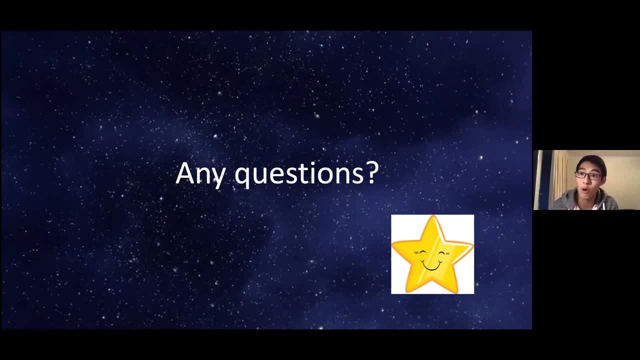 When it comes to choosing a telescope, of course, you shouldn't just go for um, you shouldn't just go for the brand. obviously, you must do even more research, like you should check if it's portable, Okay, If the size is good enough for you, if it's not too expensive. all these other factors. 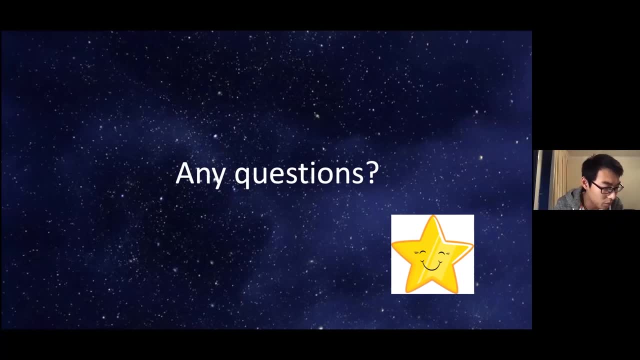 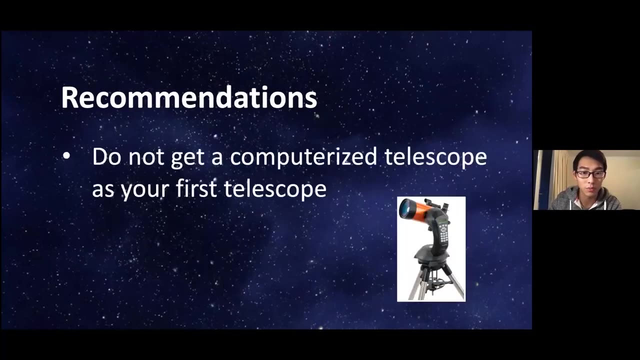 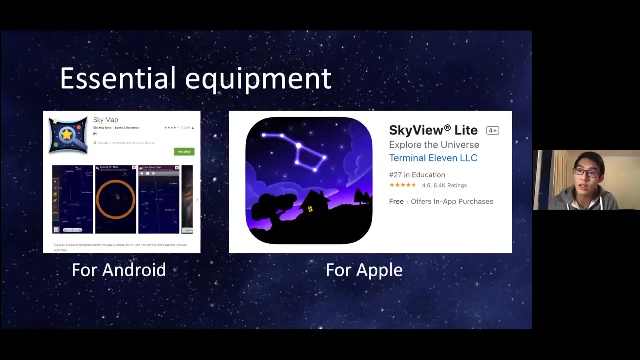 that you should consider as well. Okay, Um, someone asked about phone apps and, uh, any recommendations? uh, let me just go back to the slide, So yeah, so, as mentioned, uh, these two are the more popular apps that are used for um, 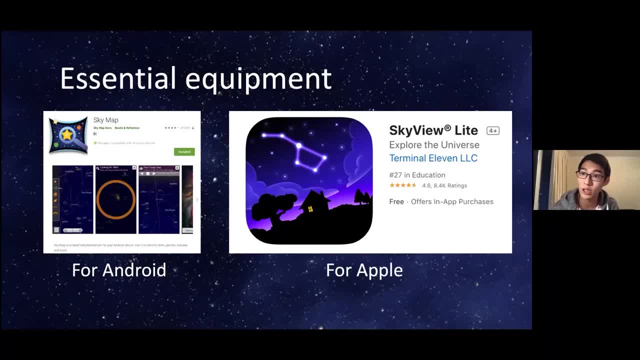 stargazing. You have um Skymap for Android users As well as, uh, Skyview Lite for Apple users, So, um, I'm pretty sure there are more apps out there on the, on the on the app store. 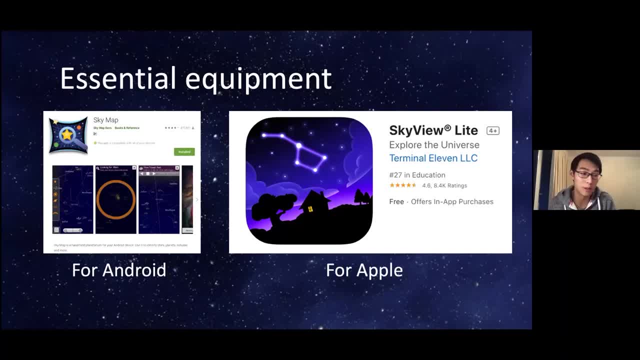 Um, but these two are just the ones that I know that are the most popular. Okay, Um, so what about a telescope where a camera can be attached? Yes, So actually, when it comes to astrophotography, I know I didn't really talk about this much- 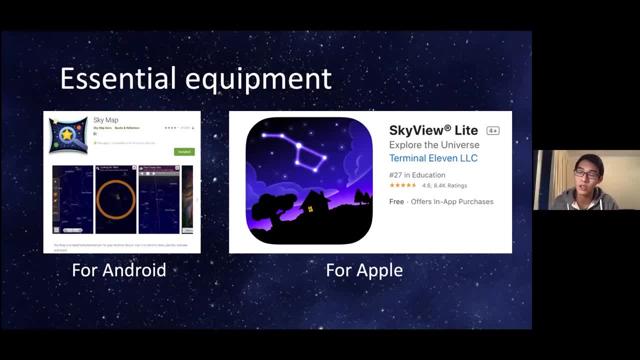 When you want to do astrophotography, you need an adapter. This is called a T-ring adapter, So it's, uh, something that you put in front of the eyepiece, or you remove the eyepiece, you replace it with the T-ring adapter and you can actually put, you can actually install. 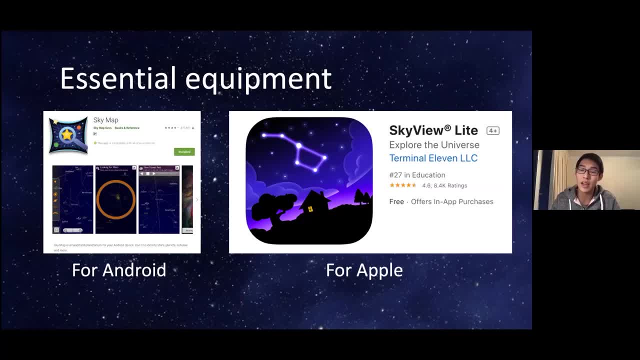 a DSLR or even a CCD camera on top of it And that allows you to capture images of the things in space? Um, but I would. I would just like to point out that I'm actually not a very experienced astrophotographer. 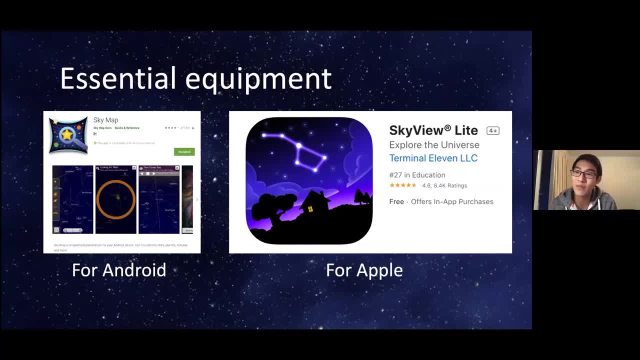 Actually, I've never done much Um. the only times I've used it, done some astrophotography, is when I've borrowed some cameras from my friends, and I don't really have much experience in that. Yeah, Okay, Yes. 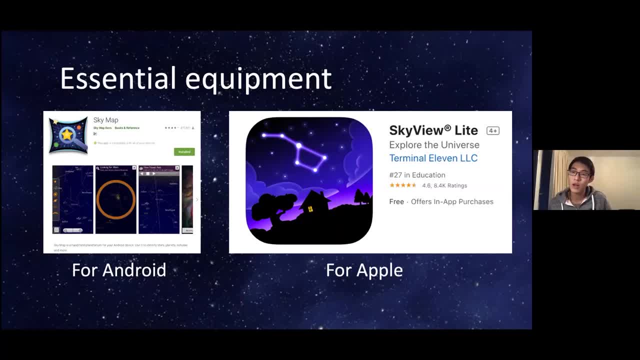 So I actually mentioned about um phone apps, like, just just like this one, but there's actually another one which is pretty popular, Um in if you are using a computer, uh, one of the apps that I, or one of the stuff that 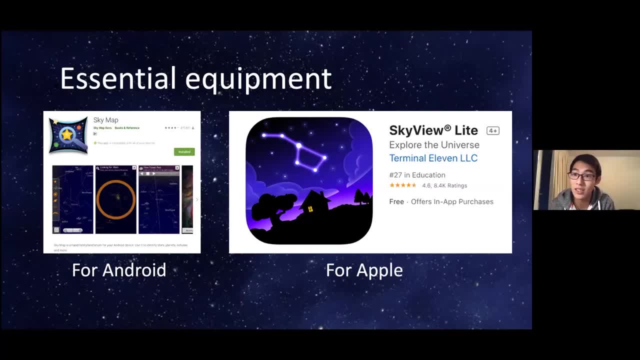 I use when I'm using my laptop is actually Stellarium. Stellarium is actually a software that is a planetarium software that allows you to see the stars in at a particular location and a time. So, um, it's the good thing again, it's free. 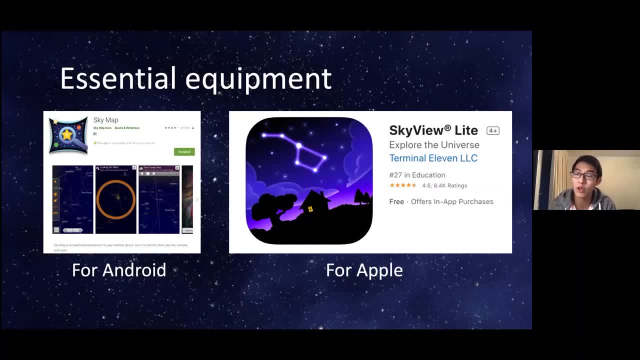 You can simply just go onto Google and just type Stellarium and you should be able to download the software into your into your computer. It's really easy to use And, yeah, I had a lot of fun playing with it, Hmm, Okay. 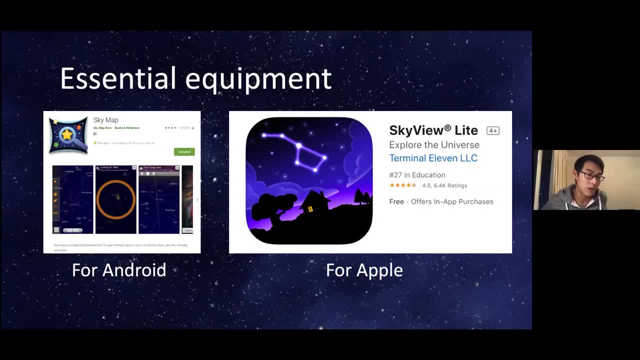 What is the best way to find amateur astronomy clubs in Sydney? Uh, unfortunately I I'm not very familiar with that because I I'm I'm from Canberra, So, uh, I don't think I can answer that question, but I'm pretty sure there are many astronomy. 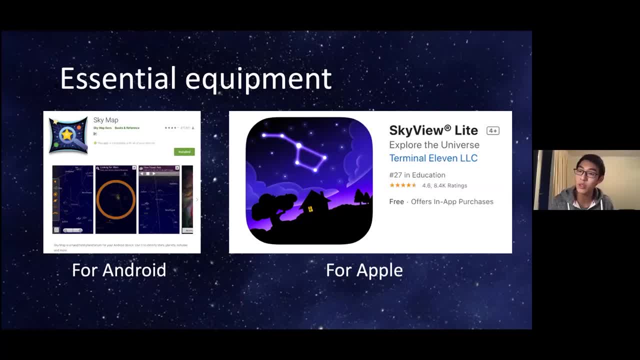 clubs in Sydney. Some of them would be part of the schools, Some of them will be part of, like, community clubs and things like that. Um, you might just have to um go online and try to find them. Yep, Okay, 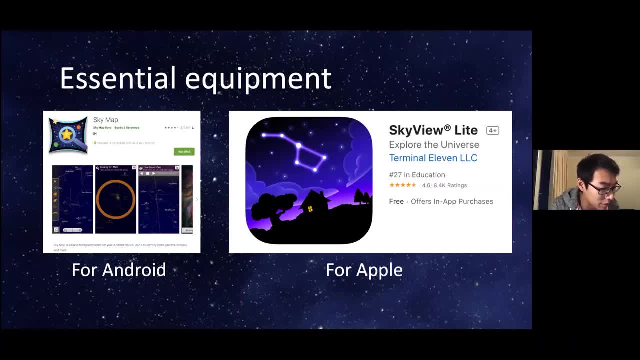 Can Dobsonian telescope mirrors um misalignment be fixed without taking to the shop? Yes, it can. So Dobsonian telescopes are actually a type of reflector telescopes, as mentioned, And the thing about Dobsonians or reflectors is that they can be um misaligned due to. 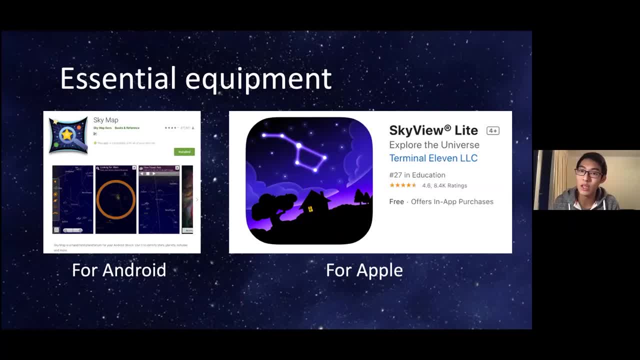 the, the mirrors and the process that you need to do to actually correct this misalignment. It's actually called collimation, So collimation it's. it sounds a bit complicated, but once you actually follow the steps it can be quite easy. 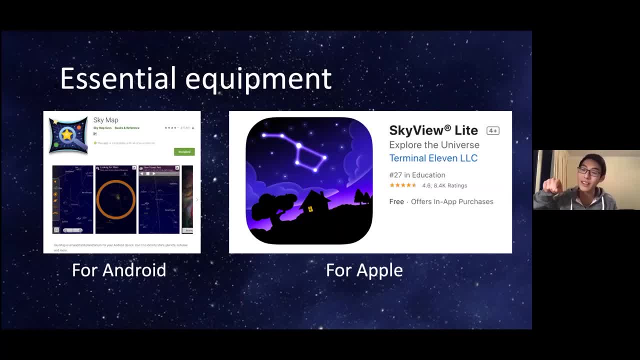 So what you do is that you use a laser and you try to align the laser as it reflects off the mirrors and try to make sure that it stays at a certain point. So by using the laser as a guideline, you can actually turn some screws and to to adjust. 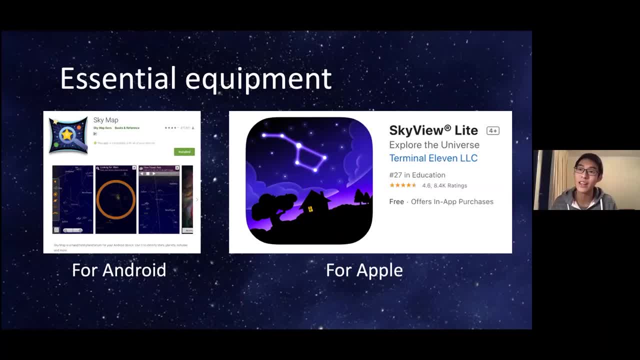 the mirror so that the two mirrors become aligned. Yeah, And that is one way that you can fix uh uh, misaligned Dobsonian without taking to the shop. Yeah, Okay, Can you use a power device to run a computerized telescope instead of using a battery? 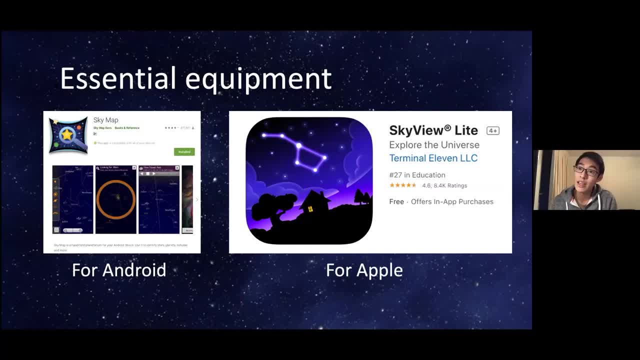 Yep, Yes, you can. So, um, I'm not. I can't remember the device on top, on the top of my head, but it's actually a power bank. So it's like you know how you have power banks for your um, you have power banks for 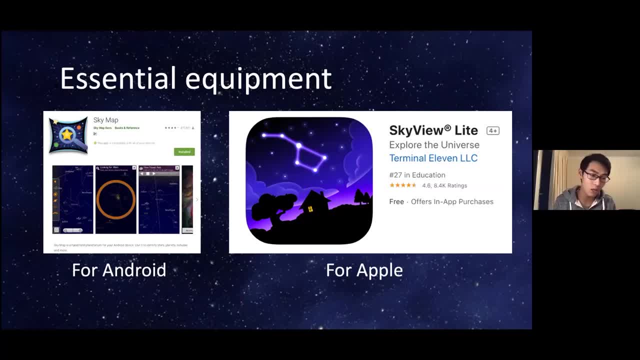 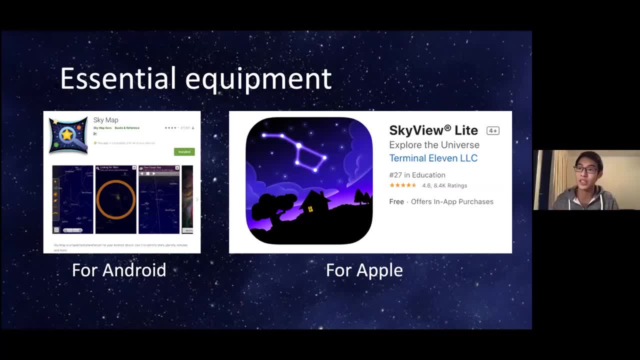 You can actually use it to basically last for your entire night of stargazing without actually having to change the batteries. Will it be a good idea? Okay, Sorry, Next question: Will it be a good idea to start with a binocular filter? 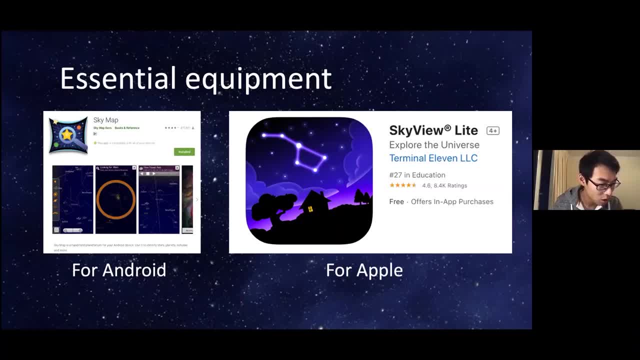 Yeah, That's a good question. Yeah, That's a good question. Yeah, That's a good question. Yeah, Will it be a good idea to start with a binocular first, before spending money on telescope? Yeah, Um, definitely. 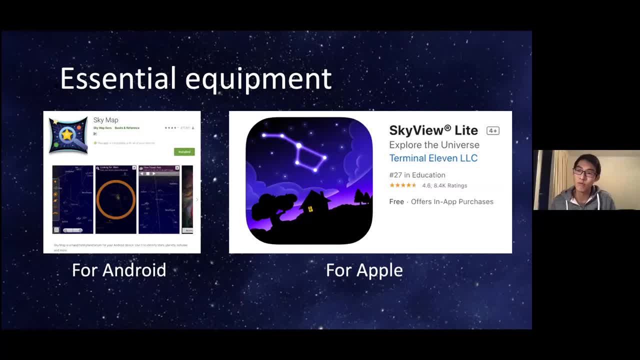 Um, especially if you think that, um, you are still maybe too young or maybe too inexperienced to to use the uh you to use a telescope, is definitely advisable to use a pair of binoculars first, because I think the good thing about binoculars is that you don't actually um 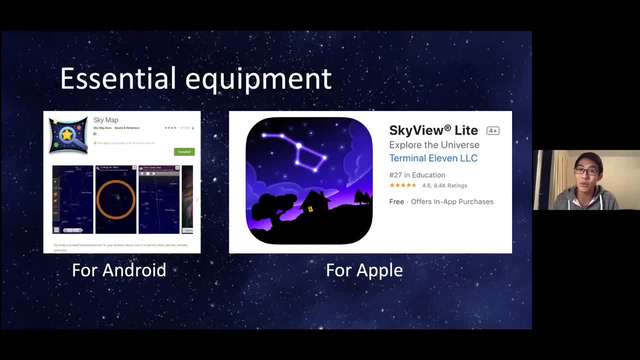 need much There. there isn't really like anything to learn. You just have to pick it up, You just have to look through the eyepiece and maybe just learn how to focus the binoculars. And there you go. You can actually use it for your stargazing trip. 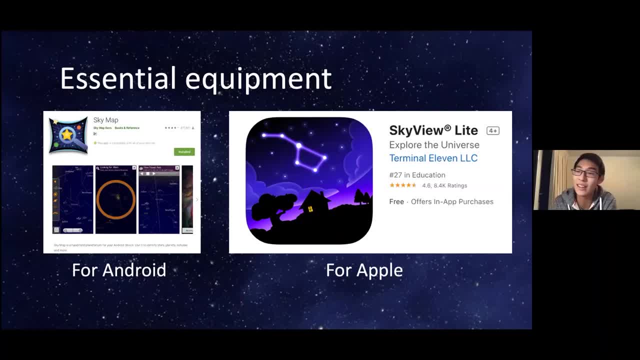 So it's really really easy to use- Definitely nothing like, uh, using a telescope- and and the good thing is that you can even get a good pair of binoculars for maybe about like $50, 50 to a hundred dollars. you can. 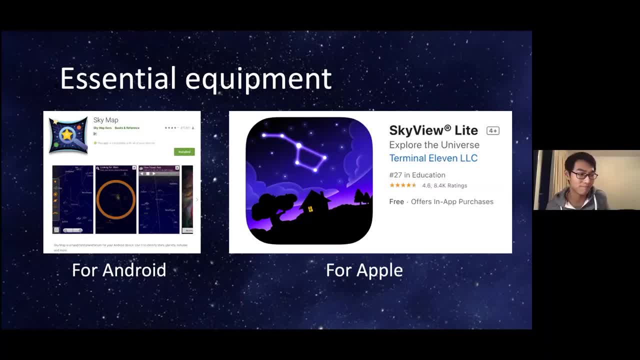 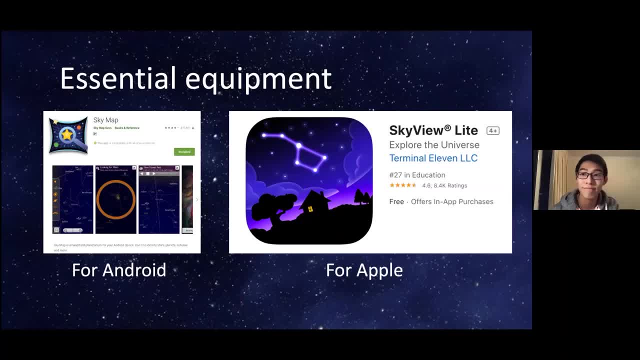 more. Okay, Um, Okay, okay, um. one more question: how do you properly maintain a telescope? um, yeah, good question. so i think for the teleth, for telescope, if it's possible- i would say it's only if it's possible- um, the best is actually to keep it in a location with low humidity. so the reason for this is: 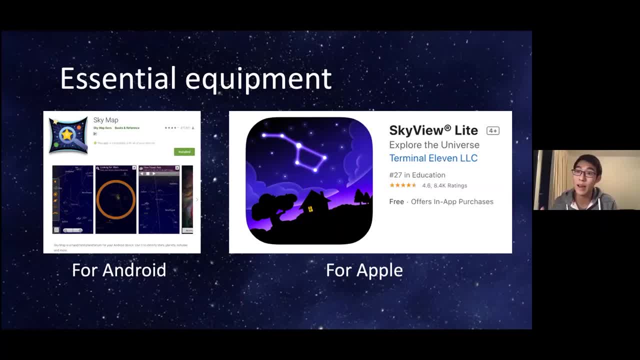 because that when you store, let's say, like a camera or even something with lenses in high humidity, the risk is that you might actually develop more or things on on the on the surface of the lens, which can be really hard to clean. so it's very important that you keep these. 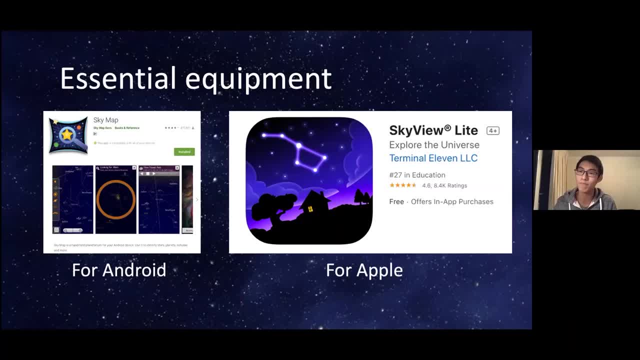 telescopes in a low humidity place and also try to um, every once in a while, give it a good wipe, yeah, so that dust and and things like don't accumulate. and the same goes to the eyepieces, the eyepieces which you use to observe, which you attach onto the telescope. remember to keep them. 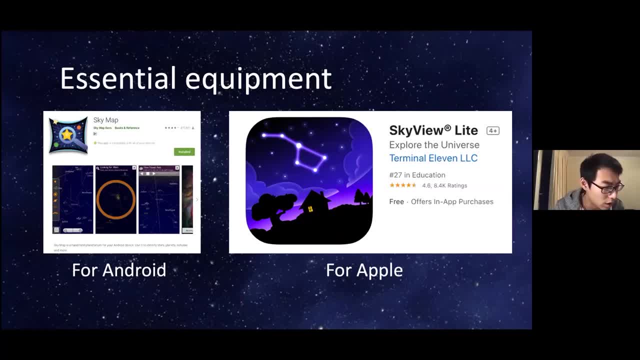 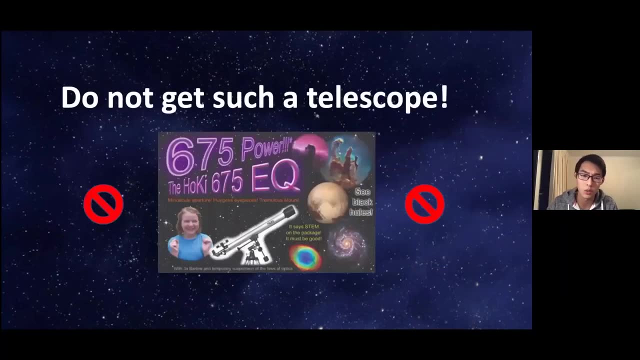 properly as well. okay, another question: what's a good brand of binoculars? um, a good brand of binoculars would also be, uh, the ones that i mentioned for telescopes such as celestron, meat and orion, and sky watcher as well. yeah, yep. 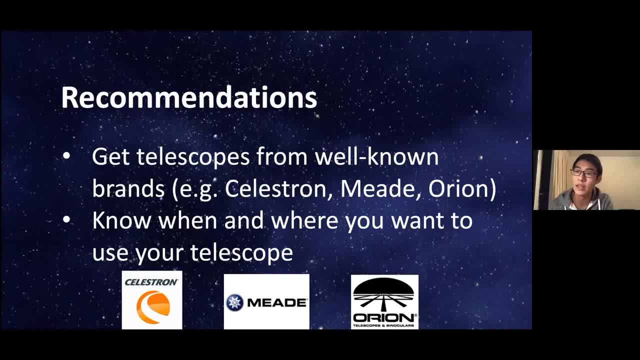 what are the best focal length eyepieces for a basic telescope? okay, um, good question. um, so it this one? um, i'm going to go a bit technical here. um, the focal length of eyepiece basically determines the field of view, as well as the magnification. 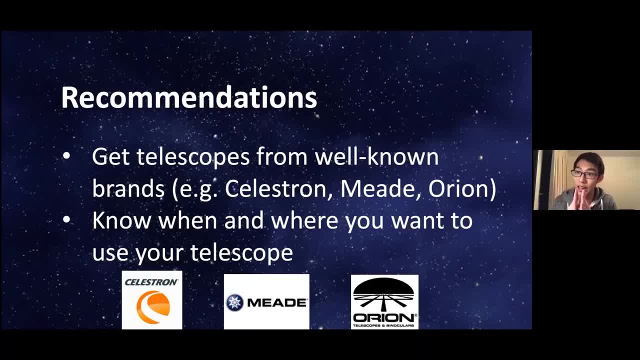 so if, let's say, you have a smaller focal length, you will get a larger magnification, if you have a larger focal length, you will get a smaller. um, sorry, if yeah, if you have a larger focal length, you. okay, i think i'm yeah. so basically the focal length affects the magnification and if you increase, if you increase. 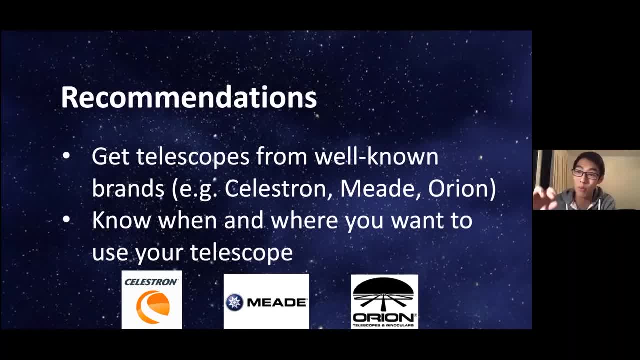 get a larger field of view, and if you decrease the focal length, you get a smaller field of view but a larger magnification. so it really depends on what you want to see. if, let's say, if you know that the object that you're observing is very small, you probably need a smaller focal length so as to 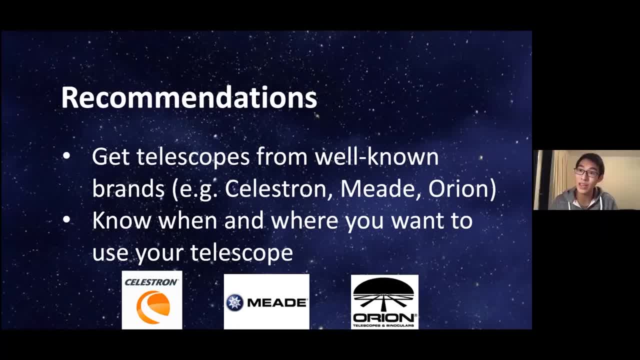 increase the magnification to view the object? yeah, but if you're looking at something as big as like, let's say, a star cluster or a andromeda galaxy, a big object, then it's advisable to use a larger focal length, which means you get a lower magnification and a larger field of view. 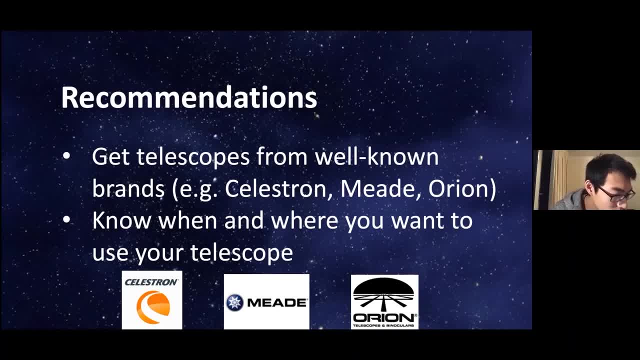 okay, um, so the other question, the next question is: every time i use binoculars, i can't get them to focus and i have to close one eye to see them through, see through them even, and then everything is always blurry. and any tips for that? yeah, um, 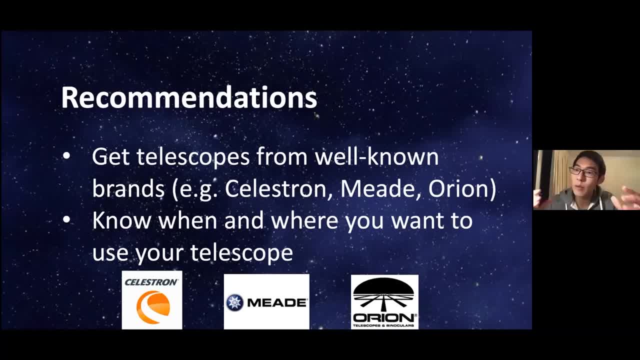 so when, when you're using a pair of binoculars, there's always some calibration that you have to do before you can use it properly, um, one of the things that that that is actually one of the the ways to actually calibrate your the pair of binoculars before you actually use it, because 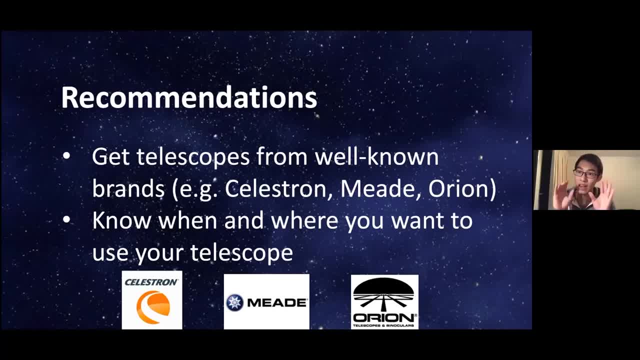 you know that you need both sides to be at the right focus. if one side is is not focused and one side is focused, you'll definitely get an unpleasant viewing experience because you can't get both to view at the same object properly. so that is actually um, that is actually one way. so 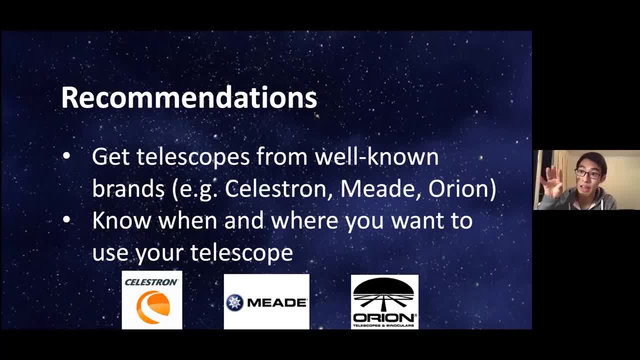 what you do is that you cover one side of the lens. there should be, uh, there should be- one side which allows you to focus the the one side of the binoculars, uh, individually, and that allows you to make sure that both- both sides of the binoculars are focused correctly. okay, um, can we see sickness from canberra during? 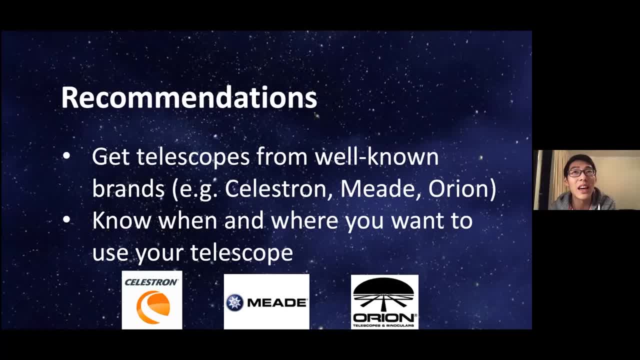 the winter. uh, winter you mean like june, june, july, right? so i'm actually not very sure. to be honest with you, um, you probably have to check um with the, the stelerium app for this, but i'm pretty sure i don't think you will get a very good view. yeah. 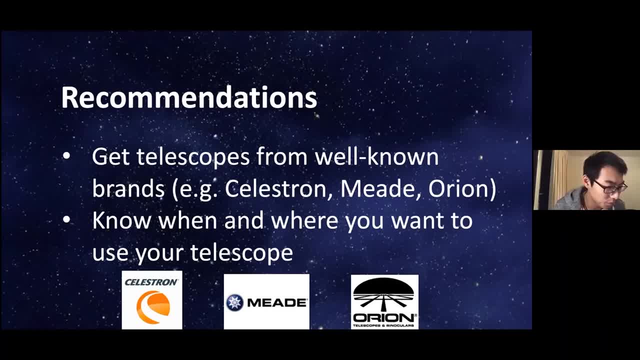 you might have to check the stelerium app. okay, is so. the next question: is a power bank better than a single battery? how does a power bank work? yes, so, um, the thing about a power bank is, as mentioned earlier, it's like using it for your phone. you can actually have um it, basically. 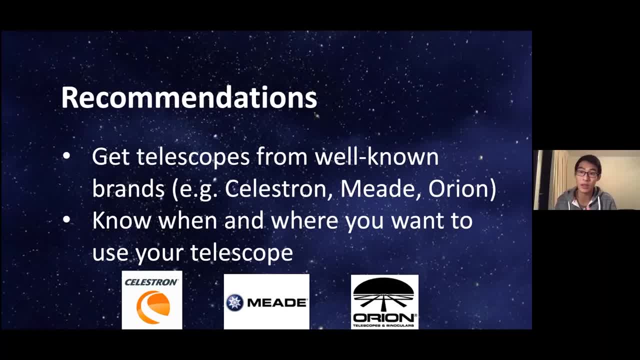 stores much more, has a bigger capacity than as compared to just using individual batteries. so with a power bank, what you do is that you, there's a wire, that which you can connect to the telescope, and, um, yeah, it basically allows you to use the telescope for, like, at least you know more than. 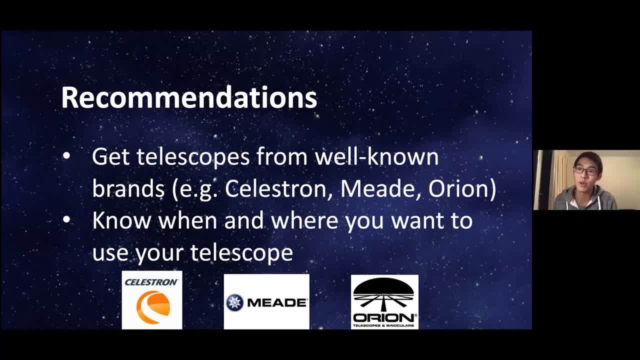 five, six hours, but whereas if you just use a set of batteries, you can only use it for about maybe 30 minutes to, at most, one hour. yeah, it's very, it's quite um easy to use. okay um, what are some interesting objects we can look forward to see in the winter? right um seems? 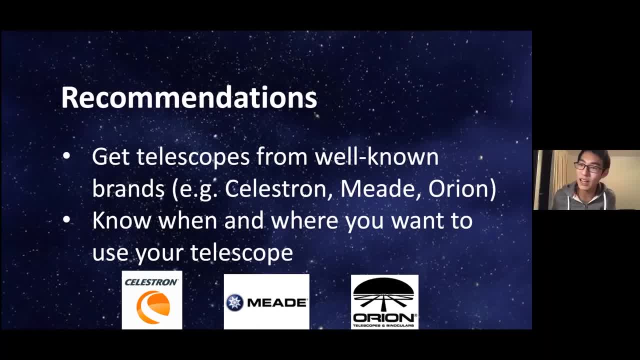 like. this is a question which um, which is pretty common um. so i don't really have um like interesting objects, in particular in winter, but i do know um. at this location in canberra, or even in australia at this time, the things that we can observe well would be the southern cross. 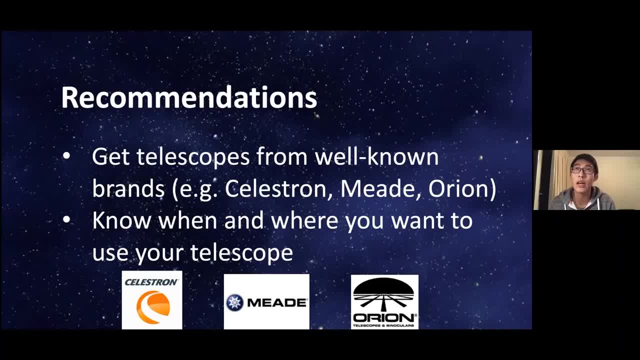 as well as, um, as well as the milky way, milky way and also, um, probably maybe sagittarius. yeah, yeah, you can observe sagittarius, but i would say that if you want to observe sagittarius, you probably have to wait for a little. a while more, not not at this time. 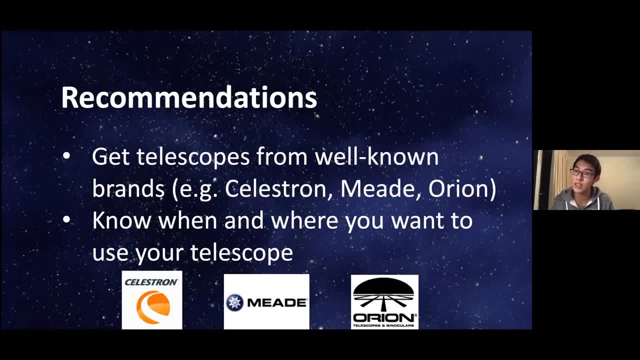 you're asking for winter, right? so yeah, sagittarius is slowly starting to rise, maybe about like 8 or 9 pm, but if you wait until um winter, it should be up like really early, okay. so another question would be: what's a good time to see saturn? um, unfortunately i do not know this. 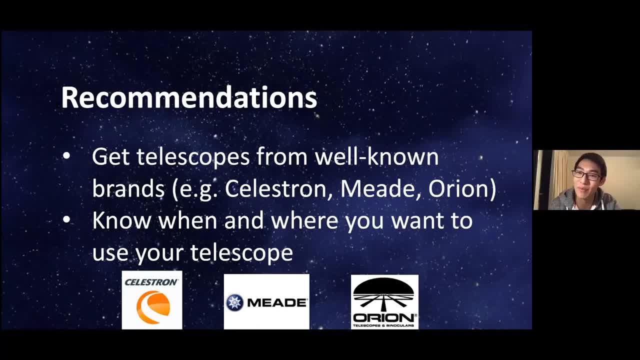 answer: uh, you probably have to check. uh, THIS IS SACRIFICE INCL. WEBIG steak culture question how canbarans see saturn. Is there any time during January to see saturn in your calendar year? the app again. um so the good thing about the app, just just to reiterate, it's a very intuitive app. 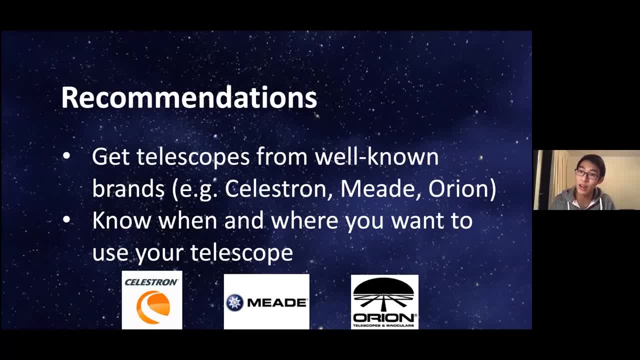 all you need to do is just input your location and time and it will tell you what all the objects you can see at a particular time in the sky. so, yeah, just just play around with it. uh, it's, it will definitely be a very fun experience to see, like what, what are the things you can observe? 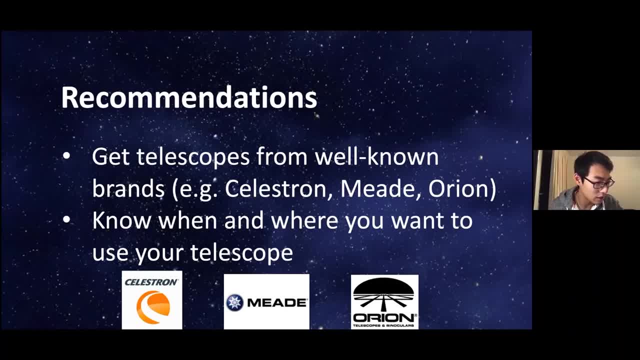 saturn, saturn would. uh. okay, someone said: oh, saturn looks better. saturn looks better from the end of june. so yeah, go go for it. um, if you need some tips on looking at saturn, i think definitely you need to have a telescope, because you wouldn't be able to see the rings and the features using just a pair of binoculars, or 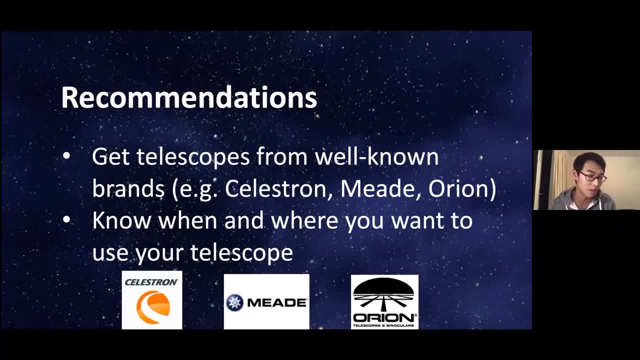 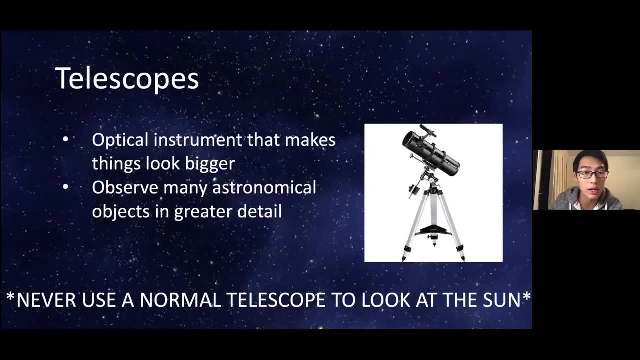 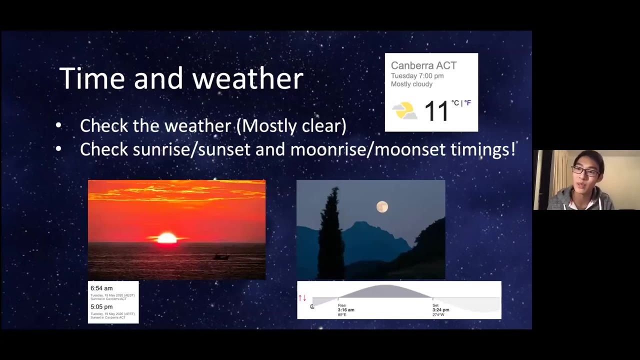 with your naked eye. you definitely need a telescope to see the rings of saturn, but what are some factors that could affect a good stargazing session? um, yes, so um, i mentioned earlier in the previous, in the previous, um, in the slides, so this: i would say this would be the main factor when it comes to your stargazing session: the time. 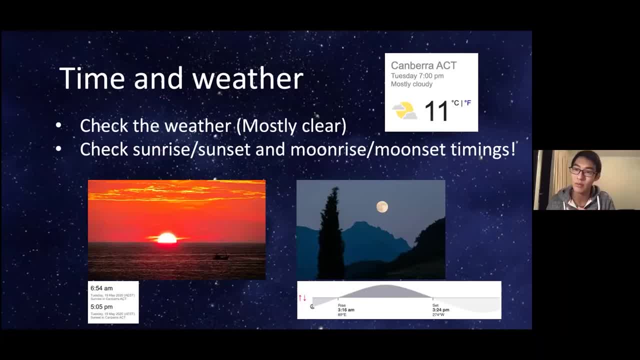 and weather, um, i would say for the in terms of whether the moon is up, uh, the weather especially, and also, um, whether they are like nearby um street lights. that is interfering with, um the stars in in the sky. so i think this is something that you have to do, your own planning and preparation. 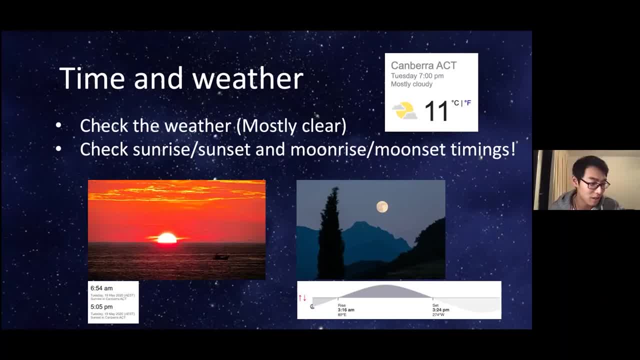 before you go out to that site for stargazing, okay, um, if not, we will wrap up. uh, thank you so much for listening to the talk uh today. um, hopefully there'll be more in the future and stay tuned for more um astro talks in the mount stromlo um facebook page. all right, bye, bye. you.